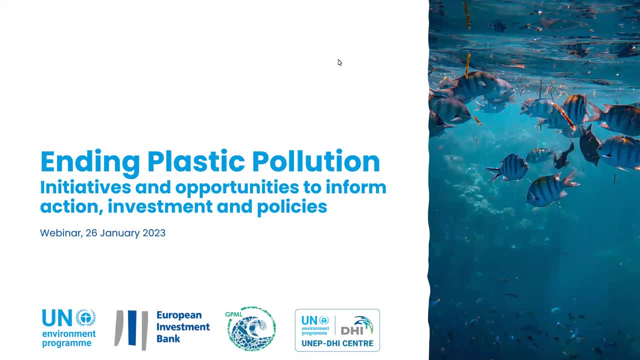 Thank you. Thank you all for joining the webinar on ending plastic pollution: initiatives and opportunities to inform, action, investment and policies. My name is Maya Bartola. I'm senior technical advisor at the UNEP DHI Center on water and environment and we're very happy to welcome you at our webinar today. 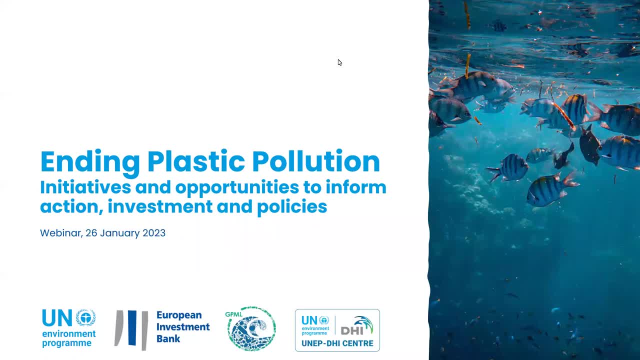 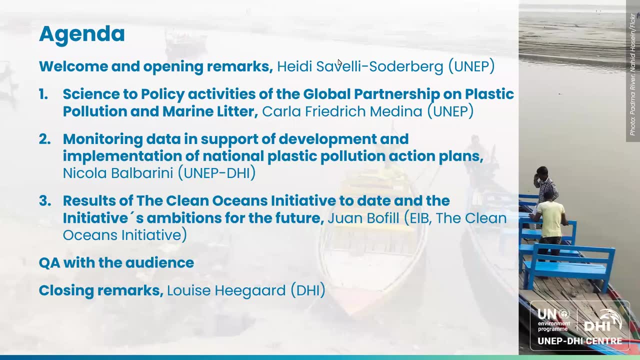 And if we could move to the next slide, please. We have a great program for you today. We'll have an introductory remarks from our colleagues in UNEP, followed by three great presenters who will speak to their initiatives and work within the plastic pollution and marine litter. 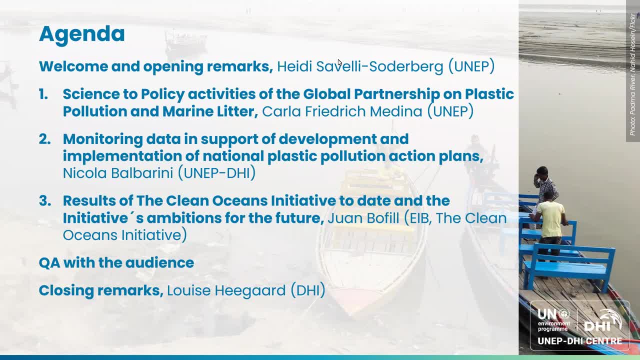 We'll also have plenty of time for the QA with the audience, So please do stay active, engage with us via chat or QA and we'll make sure to take your questions and present those to presenters in the plenary. We'll also have closing remarks by our colleague Luise and, of course, have a number of colleagues following the chat and QA to make sure that none of the questions get lost. 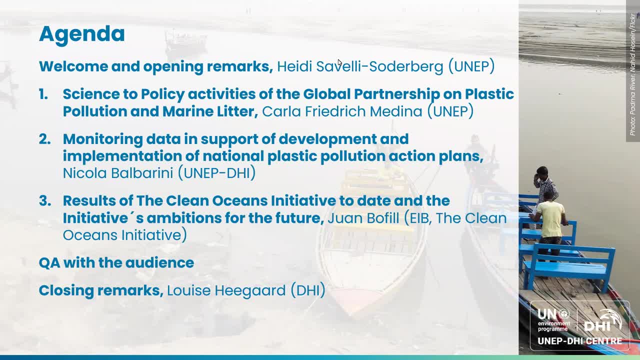 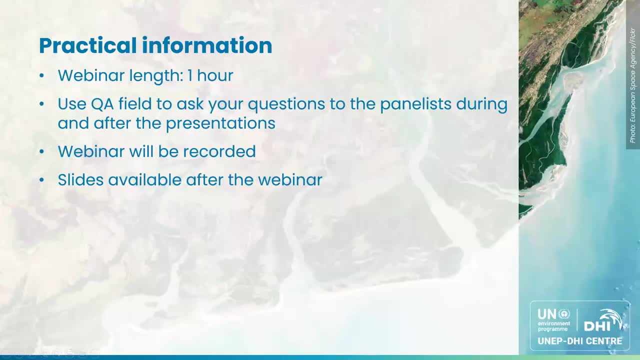 If we could move to the next slide, please. Just before we dive into the presentations, there are just a couple of practical pieces of information. We'll aim to end the webinar at 55 minutes to one hour at the very latest, so you should be able to make it for your next engagements or meetings. 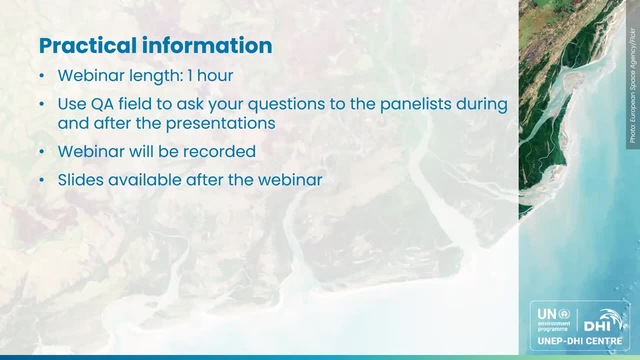 As I mentioned, we do have both a chat field and QA field- questions and answers field- where you can pose your questions, And please do so both during the presentations, if you feel you have any immediate questions, or also during the QA session. 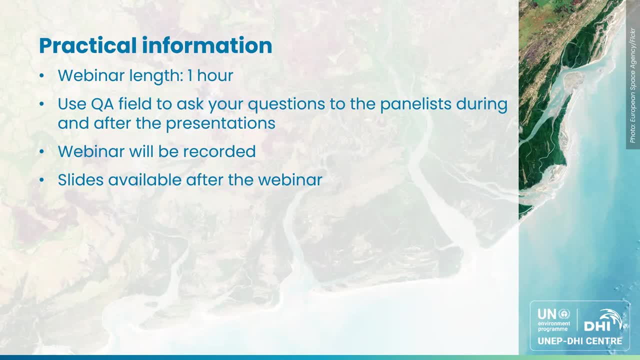 Those fields are open for the whole duration and we're very welcoming you to use those actively. Also, just a practical note: the webinar will be recorded and you and also those who are not able to attend today will be able to access webinar recording within the next week or so. 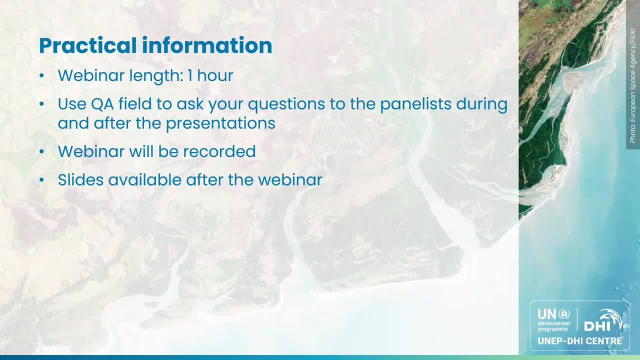 Same goes for the slides, So all the presenters Slides will be available for you for sharing and for saving after the webinar, and these should be distributed via automatic email from the Zoom platform. Now that we have gone through the practical details. 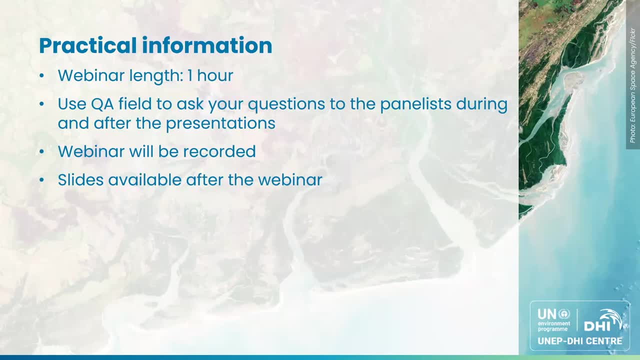 I would like to open the content part of the webinar. We'll start by Heidi Savelli-Soderberg, who will give us opening remarks. Heidi is a program officer at UNEP's Marine and Freshwater Center and Freshwater Center. 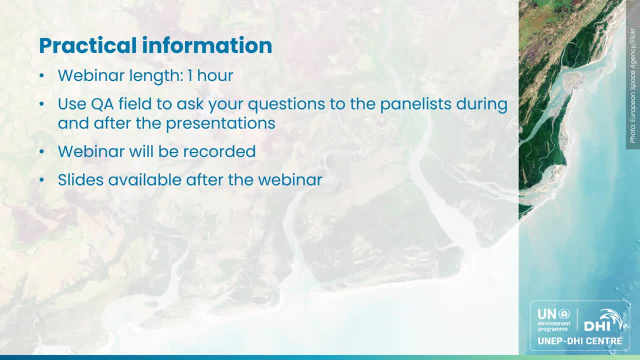 Heidi is a program officer at UNEP's Marine and Freshwater Center For the branch And if we could proceed to the next slide, I think we also have the title. Heidi holds a Masters of Science degree as an ecotoxicologist. 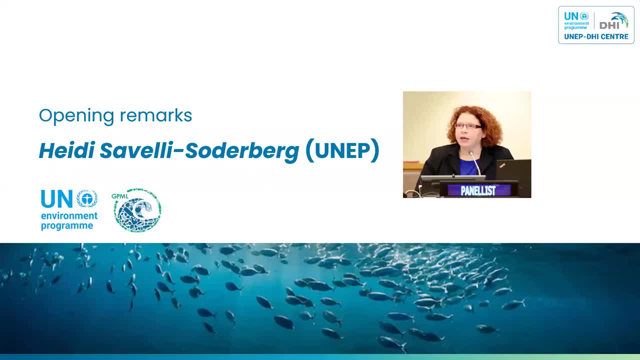 She has worked with coastal and marine management issues, including prevention of land-based sources of pollution, for around 20 years. Heidi has led marine litter and plastic pollution-related activities within UNEP since 2009.. And UNEP is the UN Environment Program. 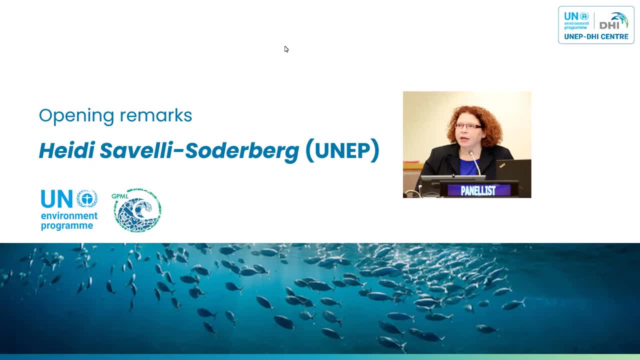 So, Heidi, without further due, the floor is yours. Thank you so much and, yes, very looking forward to the discussions during this webinar. The issue of plastic pollution and marine litter has, of course, been at the forefront of discussion since the first UN Environment Assembly in 2014,. 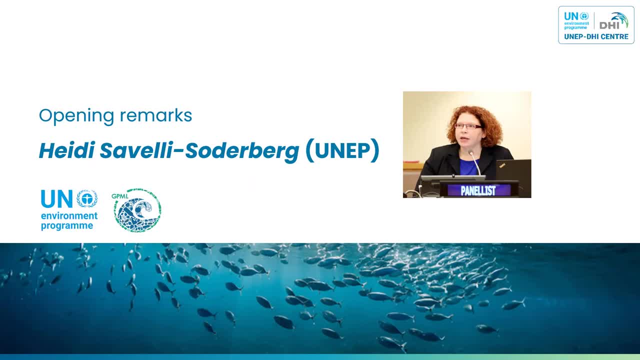 with every single assembly adopting resolutions on the topic. The most recent one was adopted now, last year, almost a year ago, and focused on a couple of different things, but more importantly, it focused on the development of an internationally legally binding instrument on plastic pollution. 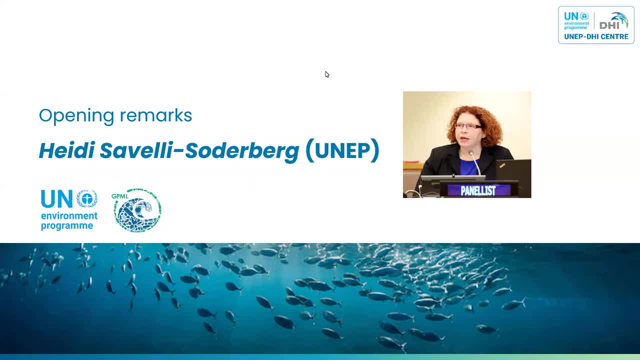 And it requested the executive director to start working on this and convening work in the first half of 2022. last year, with the first Intergovernmental Negotiating Committee being held in Uruguay end of November, early December, With the upcoming one being held in France, with more information to be provided in the website on UNEP. 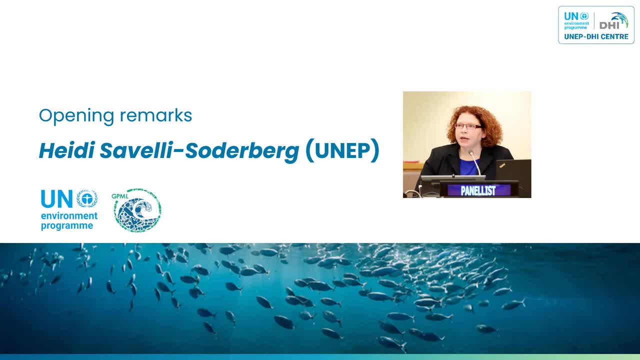 as soon as all the final decisions have been made And the work of this INC will complete by the end of 2024, and it would be followed by a diplomatic conference of plenipotentiaries to be organized in 2025,. 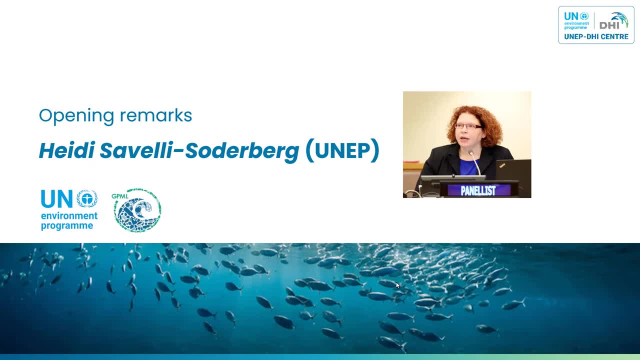 with the purpose of adopting a new policy And opening for signature the instrument that would be developed throughout this process. The resolution also requested the executive director to continue to support and advance the work of the Global Partnership on marine litter, which now is the Global Partnership on Plastic Pollution and Marine Litter. 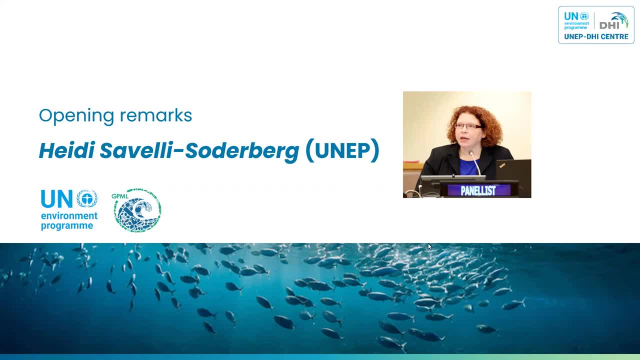 while strengthening scientific, technical and technological knowledge with regard to plastic pollution, including in the marine environment, And these are some of the areas that have been highlighted by the resolution. It also called upon Member States to continue and step up activities and adopt voluntary measures to combat plastic pollution. 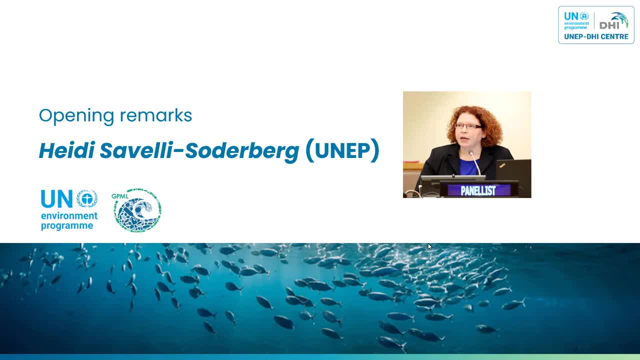 And for all action on plastic pollution. the importance of data and information is, of course, essential to inform: where would the most impact be possible to achieve and also what impact different types of initiatives and actions can have. This webinar with zooming in on exactly how to best inform action. 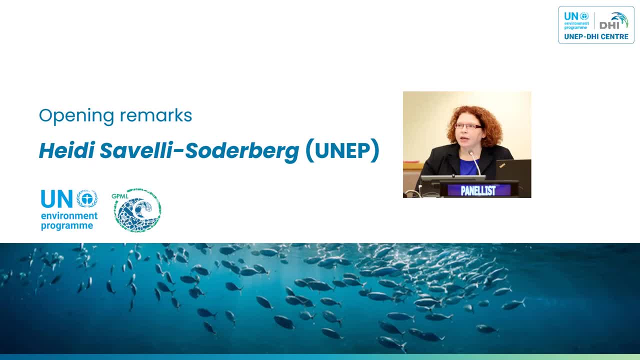 investments and policies. I will further discuss these aspects, as well as the roles of different types of partnerships and tools to strengthen such. So thank you so much for giving me the opportunity to give some brief remarks and back to you. Thank you so much, Heidi. 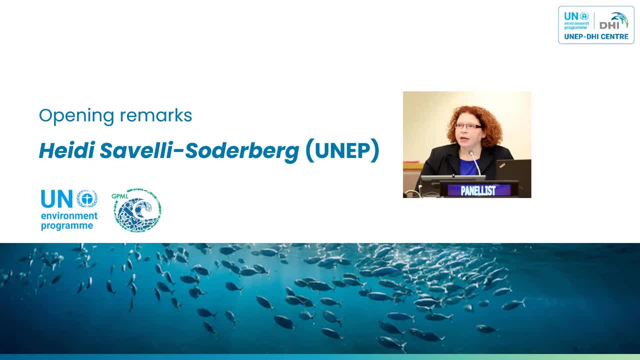 And thank you for joining us. I think this provided a great background for the webinar topic and also an excellent segue to our new first presentation of the day, And our first presenter will be Carla Friedrich Medina. Carla is Program Officer for the Marine Litter and Plastic Pollution Branch at UNEP. 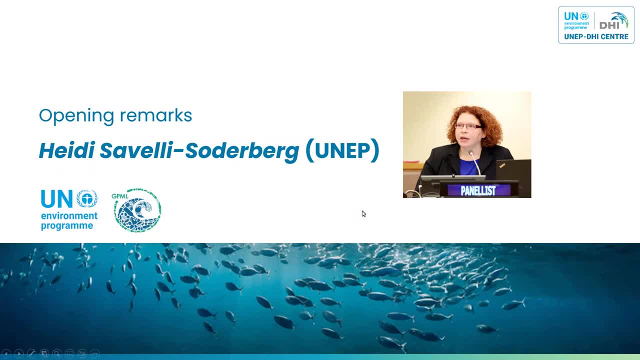 She holds two master's degrees. First one is in Conservation, Biology and Sustainable Development, and second one in International Health. Carla joined UNEP's Pollution Free Ecosystems Unit in 2021, working primarily on the marine litter and plastic pollution matters. 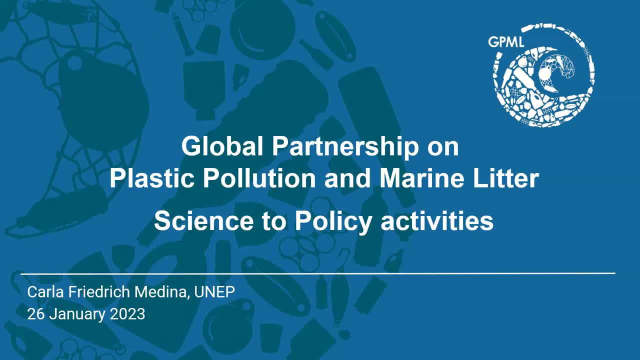 Since 2012,, Carla has been coordinating the North America Office's work on ecosystems, especially work on chemicals and waste, And before joining UNEP, Carla worked for the US Environmental Protection Agency, for the Office of Water Carla, without further ado. 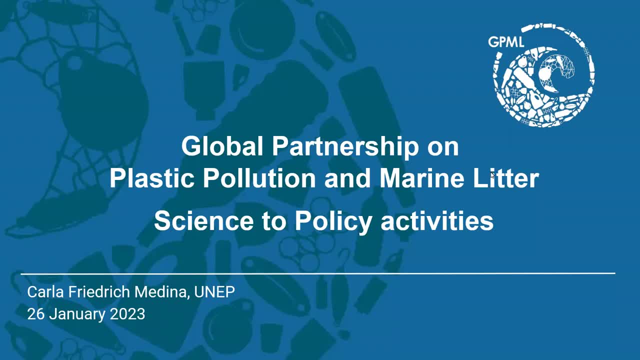 the floor is yours and I'll mute myself, and Natalie will help you to advance the slides. Thank you Great. Thank you very much, And good morning, Good afternoon, Depending on where you are. Many thanks to BHI for organizing this webinar and for inviting us to participate. 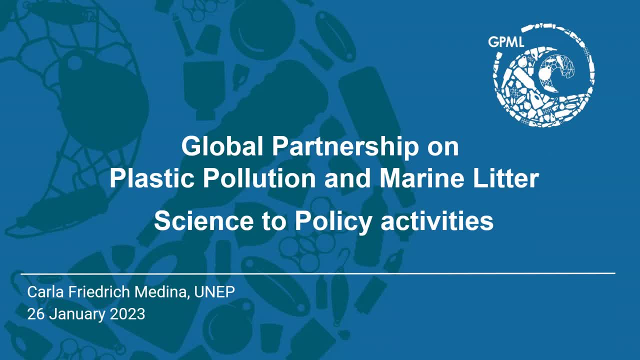 My name is Carla Friedrich Medina and I am part of the Secretariat team of the Global Partnership on Plastic Pollution and Marine Litter, And I'm based in Nairobi, Kenya. Next slide. So for those of you not so familiar with the partnership, 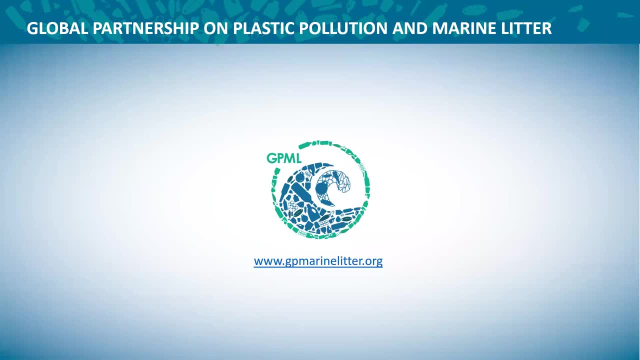 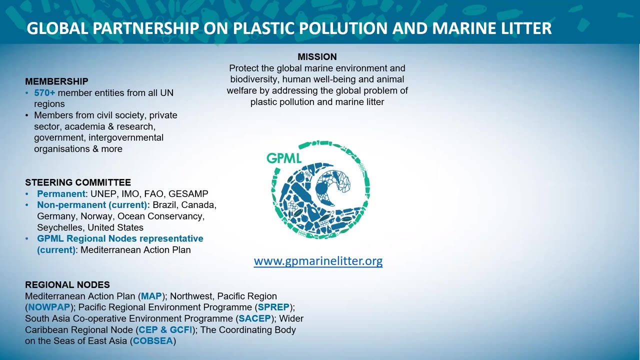 this is a little primer on the Global Partnership on Plastic Pollution and Marine Litter And maybe if you click on the next ones- sorry that it's animated- you can see its mission: to address the urgent global problem of plastic pollution, including in the marine environment. 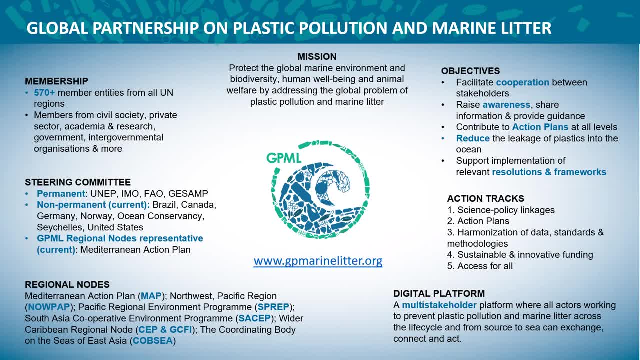 which has become so obviously urgent, And since its launch more than 10 years ago in 2012,, it has grown to over 580 member entities from more than 100 countries all around the world. It is a voluntary multi-stakeholder partnership. 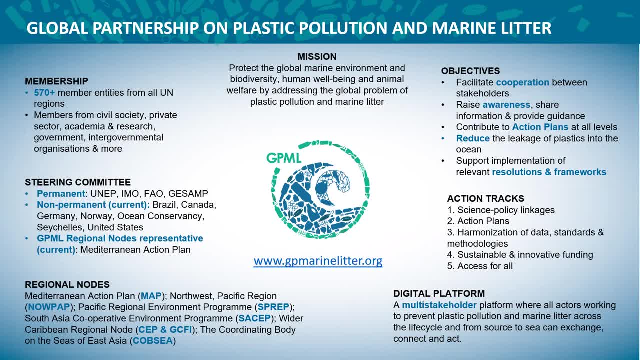 That brings together civil society, the private sector, academia and governments under the common goal of eliminating marine litter and plastic pollution. And you can see here the current composition of the steering committee and also the six regional nodes which can amplify the work. 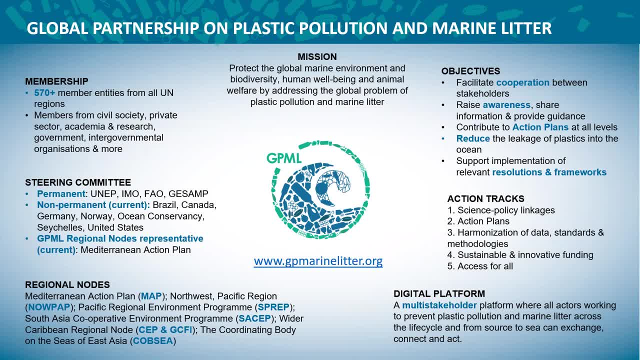 which amplify the work of this global partnership on a regional level. So the partnership facilitates cooperation and supports the implementation of relevant resolutions, such as the UNEA resolution that Heidi spoke about, but also other resolutions and frameworks from other intergovernmental entities and intergovernmental bodies, and beyond. 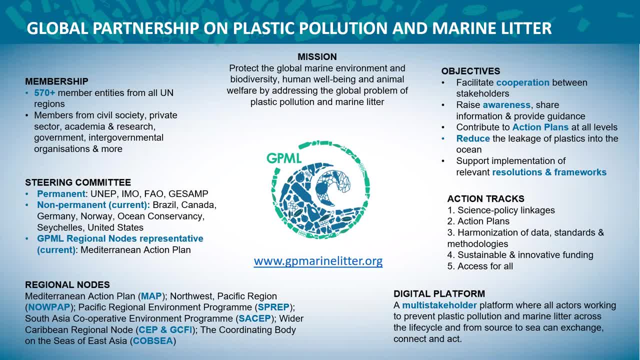 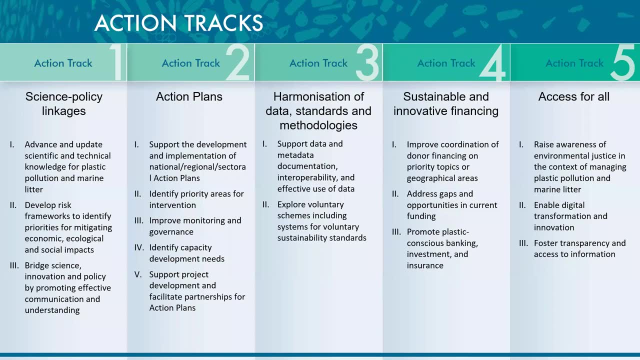 And I will speak about the action tracks on the digital platform on the next slide. So next slide, please. The partnership has been streamlining its efforts into these five action tracks to advance the many objectives that you can see here. Some of the recent ongoing activities under action track one on science policy linkages: 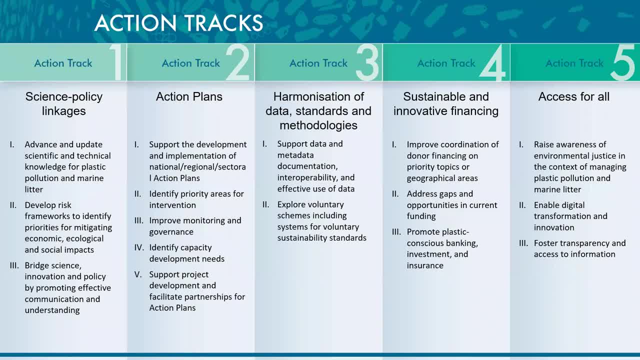 on which I'm going to be focusing a bit more on today's presentation include, for example, a series of issue briefs on topics of interest or emerging concern that were developed with the aim of to foster discussion and to make science accessible and useful to policymakers and to a broader audience. 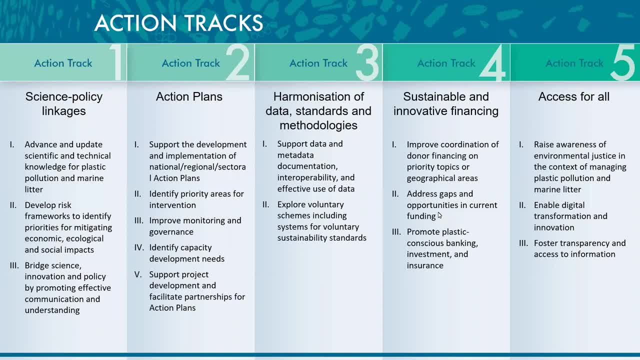 The topics of this initial series of six were: a mass balance approach to quantifying plastic pollution. unnecessary, avoidable and problematic plastics. additives and the circularity of plastics. human health and environmental impacts along the lifecycle of plastics. a risk assessment approach. 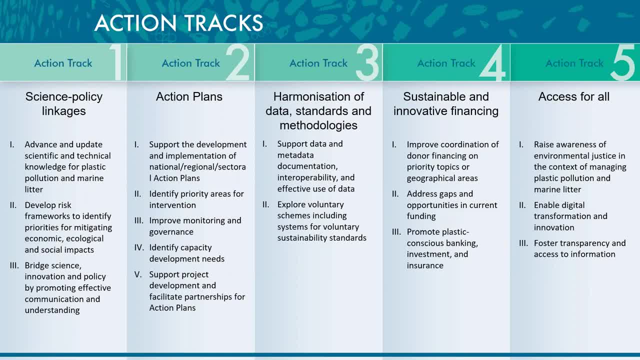 and the nexus between climate change, biodiversity loss, pollution and plastics. So these issue briefs and the series of webinars and workshops that were organized to provide opportunities for outreach on these topics were undertaken through a collaboration between the University of Georgia, Greed Arendelle, University of Wollongong and UNEP. 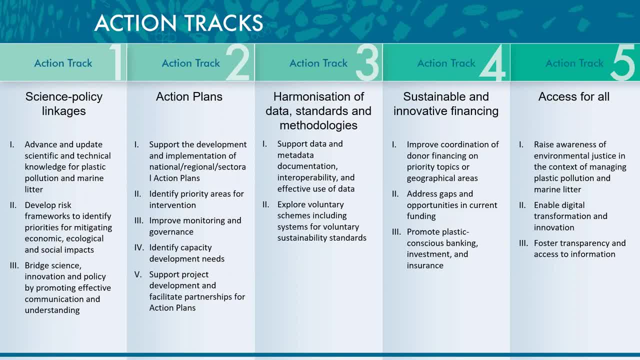 Another recent activity was undertaken by GESAMP, the GESAMP Working Group 40,, which recently convened a workshop on developing risk assessment framework for marine plastics and microplastics. It took place in Busan back to back with the 7th International Marine Debris Conference. 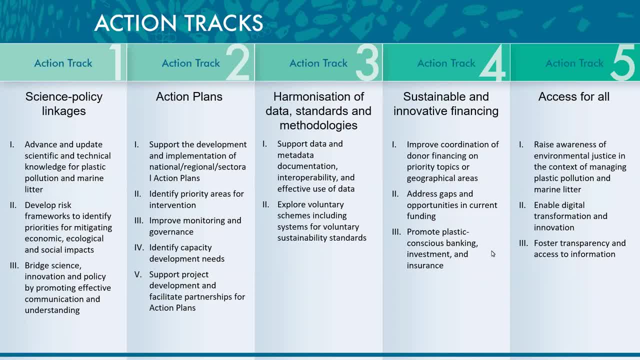 in this past September. Another example: also, FAO and UNEP have been generating reports and convening events regarding the issue of agricultural plastic pollution And through this action track, the partnership will also continue to connect with experts and gather relevant information to provide updates to the state of knowledge. 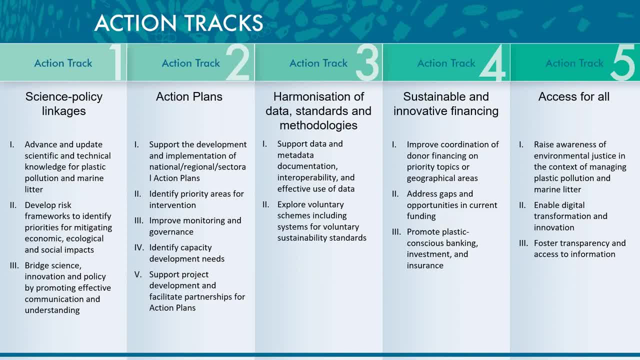 that was very well vetted and extensively peer reviewed and summarized in the From Pollution to Solution assessment, a global assessment of marine litter and plastic pollution a couple years ago. So the partnership will continue to look for effective ways to gather and communicate these updates. 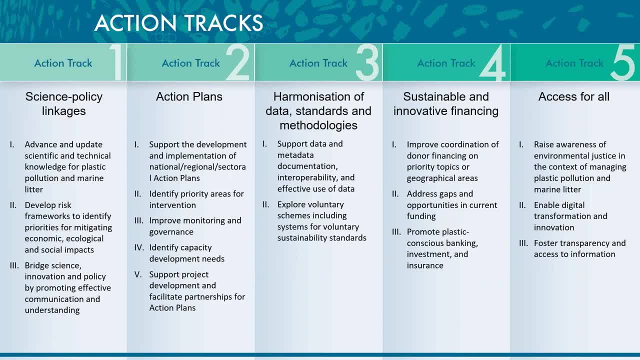 because there's a lot of science evolving on this issue and we want to stay abreast of that And perhaps we will be following something like the recent experience of the six-issue briefs and the opportunities for discussion. So the science policy action track also aims to encourage. 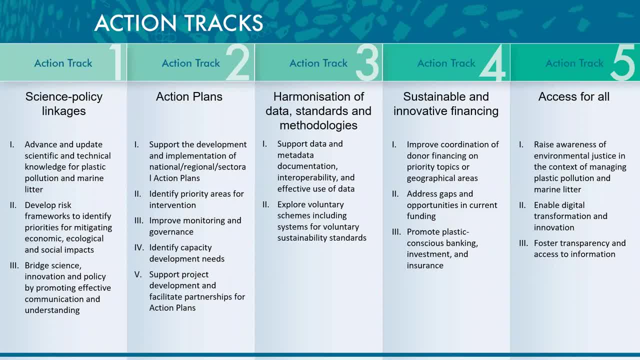 and incorporate information and experiences from citizen science. initiatives that foster effective community engagement in the generation of data and information regarding marine litter, Information regarding marine litter and plastic pollution, And perhaps I can talk a little bit about that later. I don't have a ton of time. 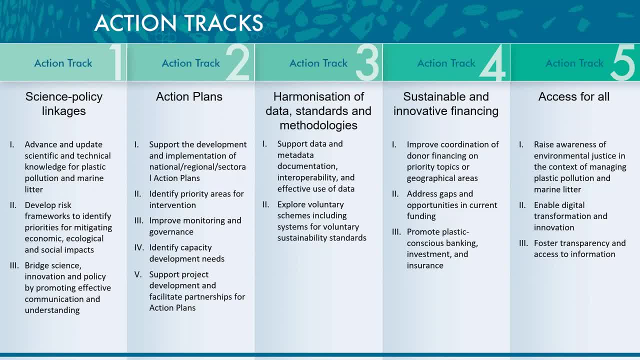 With regards to action track two- and I'll speak in much less detail about that and all the others, various members of the partnership have been engaged in supporting the development and implementation of national, regional and sectoral action plans all around the world. 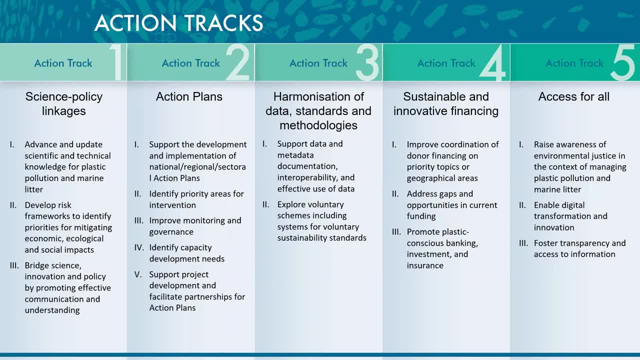 And much additional work on action plans, including the development of guidelines for undertaking a national source inventory approach to assist in action planning, is underway with support from various partners and governments, And we really hope that all this work will be useful to support the development of an ambitious global instrument. 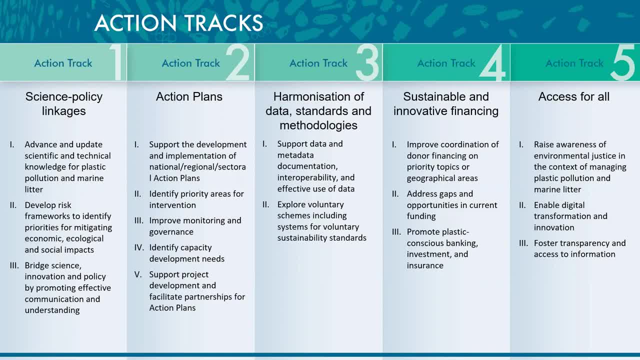 to end plastic pollution, So by countries understanding the issues and being able to establish action plans. hopefully they're also going to be better engaged in these global discussions On action track. three communities of practice on ontology and data harmonization have been established. 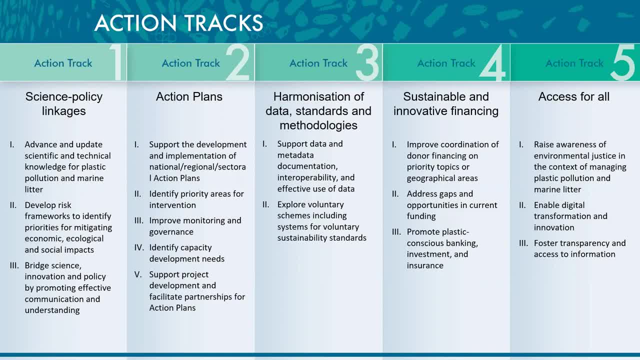 And also an expert group on methodologies and models for monitoring plastic pollution has been convened and will form an upcoming community of practice as well. Under action track four on sustainable and innovative financing, DHI has been supporting with an overview of funding modalities and a strategy to support development. 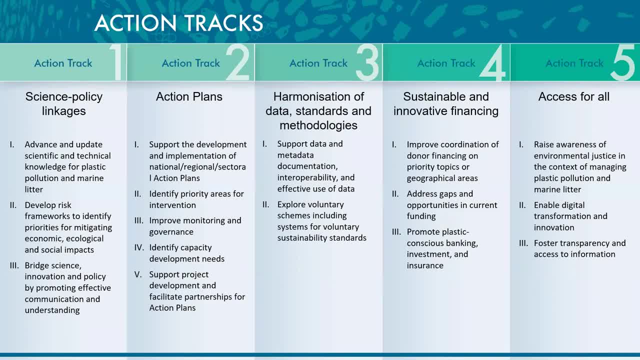 and implementation of action plans, And perhaps Nicola will speak a bit about that in his presentation. Under action track five, the partnership is working, for example, with UN Habitat on the development of awareness-raising materials and initiatives regarding decent jobs and the just transition in the informal sector. 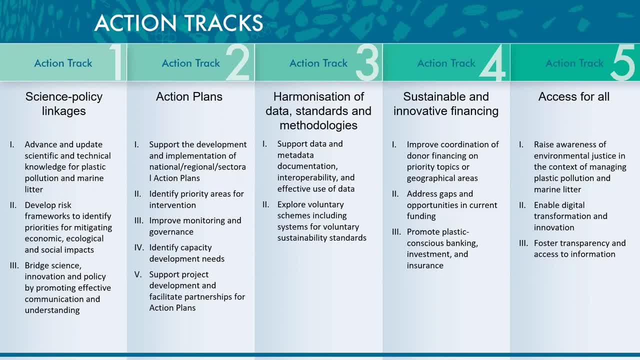 across the plastics value chain, including waste pickers. The partnership also continues to disseminate knowledge through, for example, the massive open online courses, the MOOCs and related master classes on emerging topics, And it is enabling digital transformation and innovation. 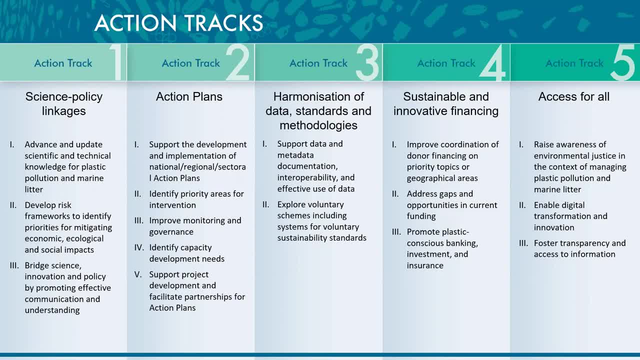 through the digital platform on plastic pollution and marine litter, which I will highlight in a minute, Next slide And this slide. I'll just very briefly say that these action tracks are very well interlinked And, you know, a key central area is the development. 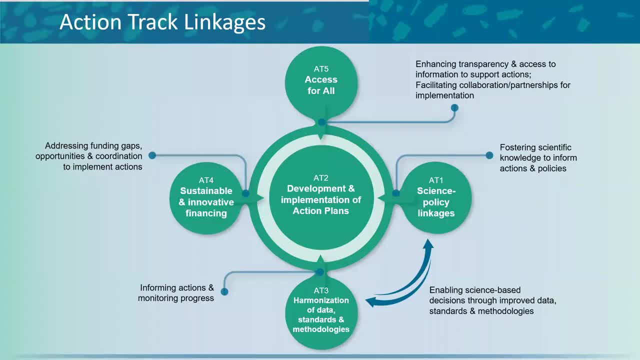 and implementation of these action plans And the other action tracks have their own work, but also are very closely related to this important topic. Next slide, And so the digital, So the partnership's digital platform, which was set up in 2020,. 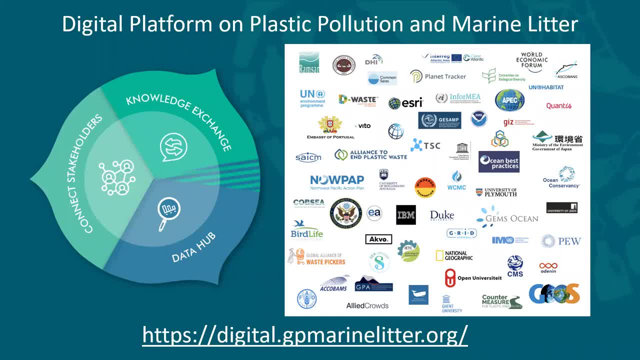 and seeks to connect and inform all actors working to address marine litter and plastic pollution. This is a multi-stakeholder, mostly open source platform that compiles and crowdsources different resources, integrates data and, very importantly, connects stakeholders to guide action. 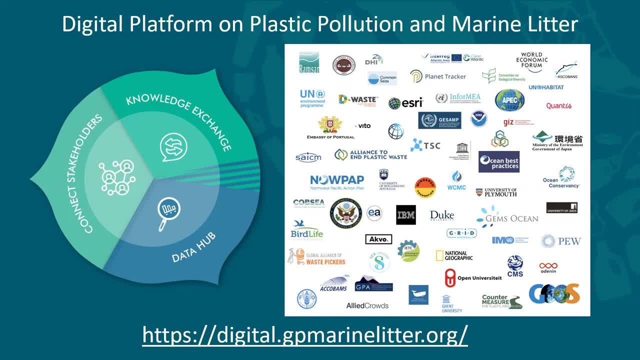 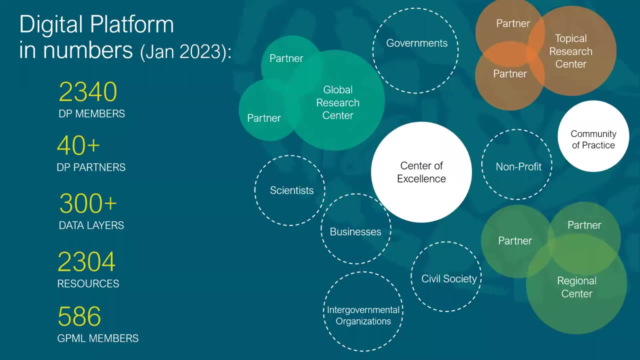 around the issues of marine litter and plastic pollution, And here you can see many, Some of the many partners that have been directly contributing to the digital platform in various ways. Next slide, please. And here is the platform in numbers. Very quickly, over 2,000 members have joined. 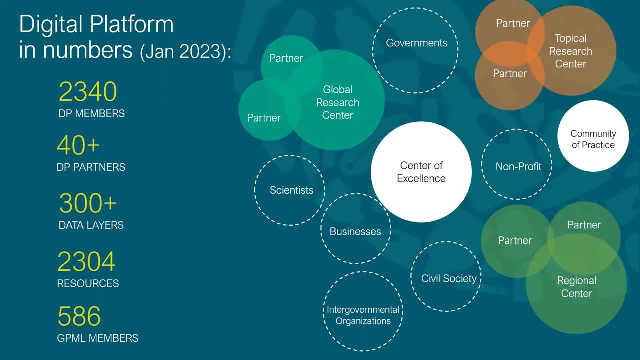 either as entities or as individuals. So far, over 40 partner entities that you could see in the previous slide have contributed to the development of the platform, including by, for example, providing all these- you know, over 300 data layers. 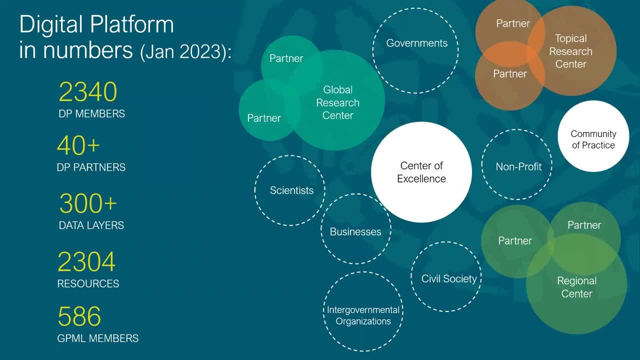 as well as many other resources And through its outreach efforts, the platform has also helped the Global Partnership on Plastic Pollution and Marine Litter grow its membership which, as I mentioned before, accounts with almost 600 entities from around the world- And these are not individuals. 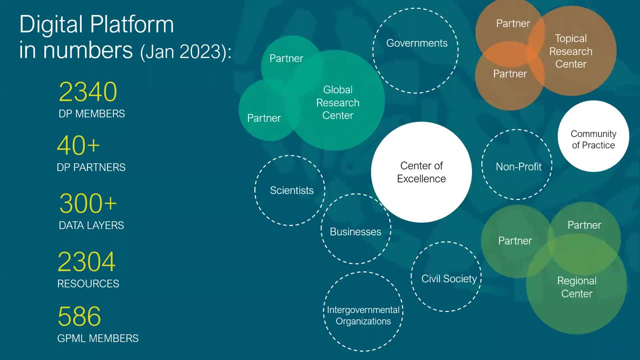 but these are organizations or governments, NGOs, businesses, et cetera. And, very, very importantly, the platform is enhancing the creation of, for example, communities of practice on key issues and regional centers of excellence on this topic of plastic pollution and marine litter around the world. 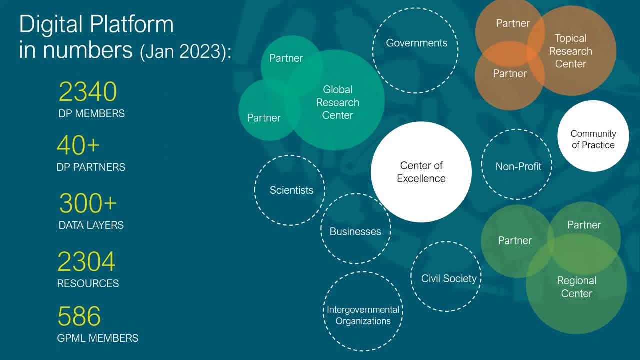 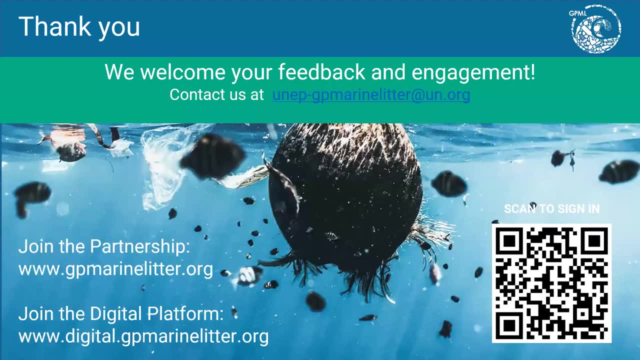 And my last slide. Thank you so much, everybody. Welcome your feedback and your engagement. Here's some of our contact information and also you can click to join the partnership as an entity or join the digital platform either as an entity or as individuals. 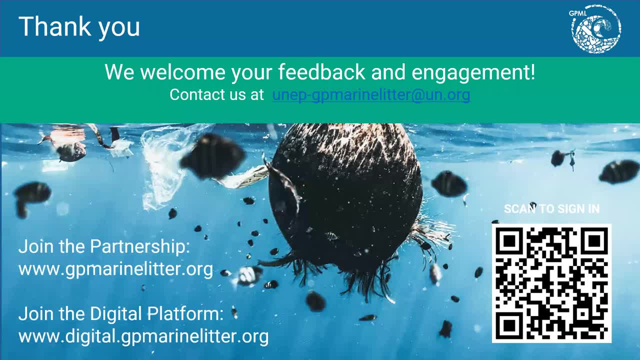 Thank you so much and I look forward to the discussion. This is excellent. Thank you so much, Carla, for this great introduction to the many, many activities of the GPML and the platform and the partners, And I think that gives us a good segue. 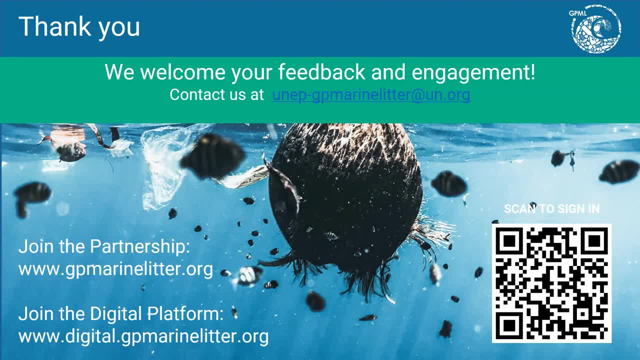 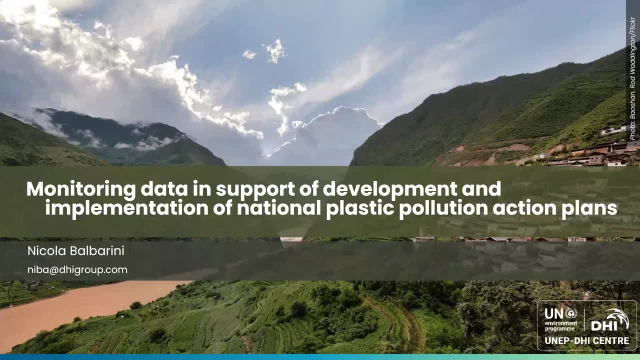 to our next presenter. Our next presenter is Nicola Balberini. Nicola is water resources expert from UNEP DHI Center. He's water resources engineer and has really played a key role in the development of a global early warning system for plastic litter in freshwater ecosystems. 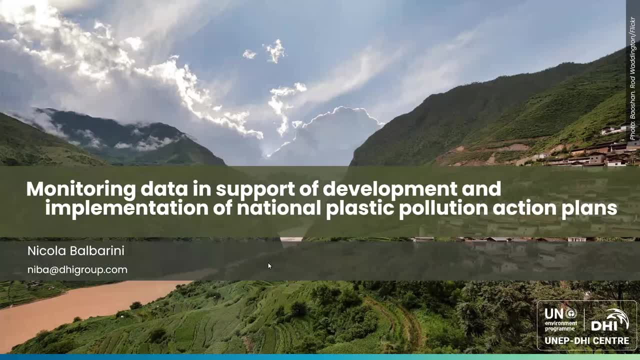 By applying DHI's technology and knowledge in various locations around the world. Nicola has also been involved in several research initiatives to address plastic pollution globally. With that, Nicola, the floor is yours and I can see presentation is already up and running. 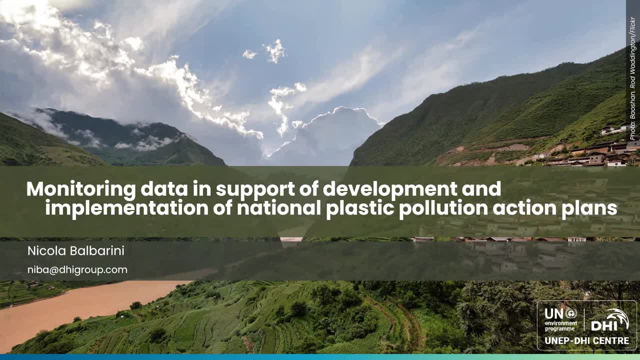 Thank you. Thank you very much, Maya, for the introduction And thank you also, Carla, for kind of like introduction to what I'm talking about. What I would like to do now is to dive a little bit deeper in some of the activities that UNEP DHI Center. 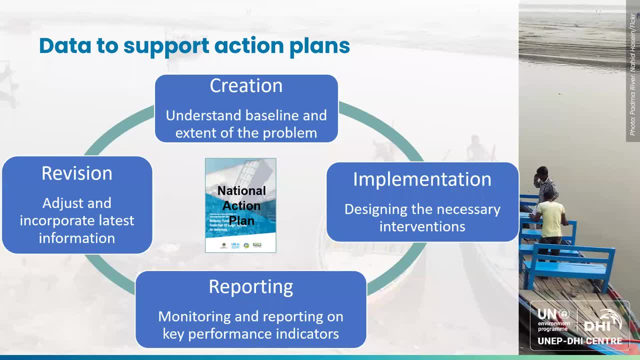 has been supporting GPML and UNEP with in relation to plastic pollution, And I think maybe a good way to phrase this is to focus a little bit around the aspects of action plans or, more in general, of planning and implementation of actions, which is an important part of action plans. 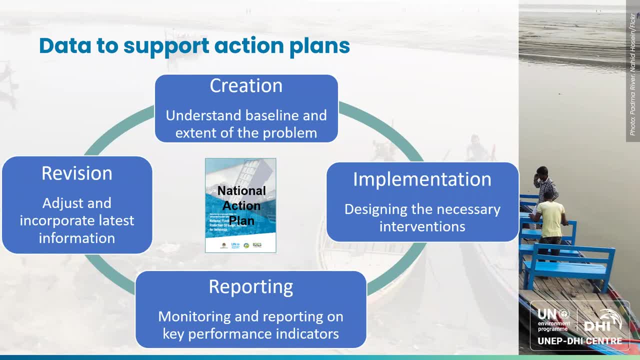 And there are two aspects I would like to walk you through, or two sets of activities I would like to walk you through in the next 10 minutes. The first one is focus a little bit more around the data and information that are required in order to make informed decisions. 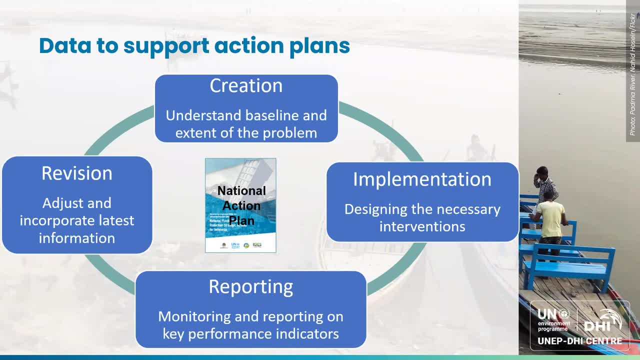 As already Heidi highlighted during her introduction, And then in the second part, I will more focus around what are the actors that are involved in order to collect and make this data available, and how are ways of funding and supporting these actors in order to ensure a sustainable implementation. 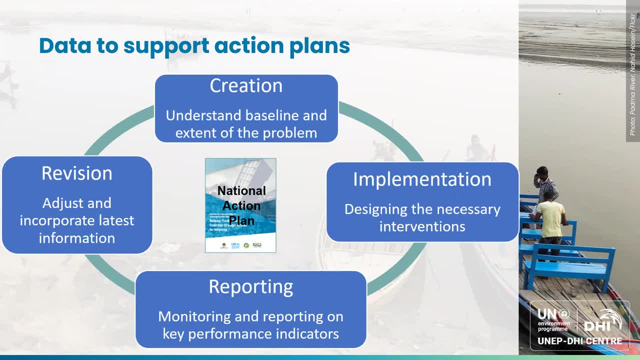 of action plans and of interventions. So if we start first with having a look a little bit of what does an action plan incorporate, What are the needs, What are the different phases of an action plan, And this, of course, can be drawn in different ways. 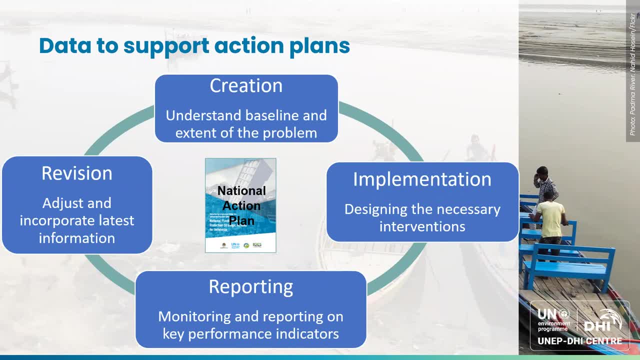 But there are four major, let's say steps, phases, that are common during the action plan, in national action plans. The first one is, of course, the creation phase. This is the part where data and information are needed in order to understand the baseline, understand the problem. 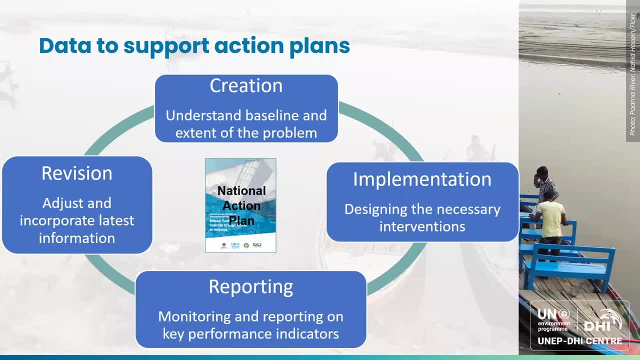 Once this information are gathered- and this is well understood- there is an implementation phase where different interventions, policies, are designed and start to be implemented. There is then a monitoring phase where progress is tracked. Hopefully, progress is tracked, And if not, then there is a revision phase where, of course, 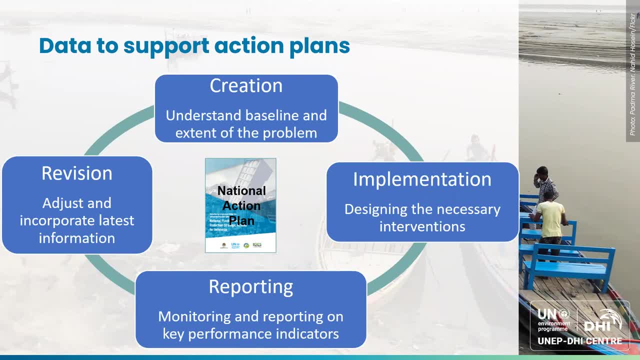 the required adjustments are implemented in the plan and in the interventions in order to ensure the successful implementation during the next round of the action plan. As you can see, data are really key, All these different phases of action plans And if we can go to the next slide. 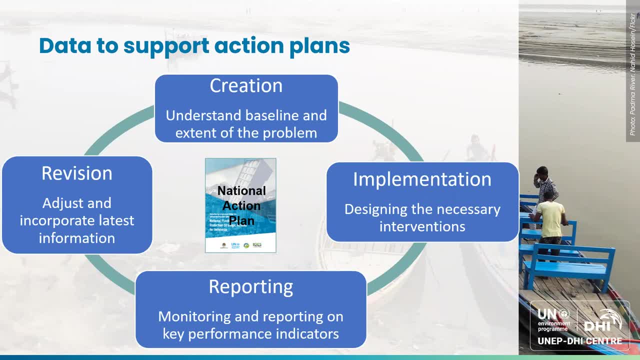 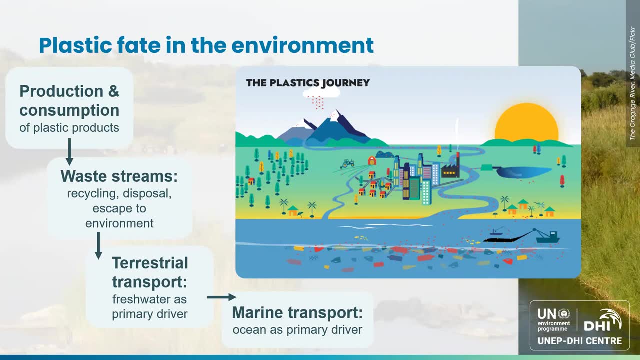 what I would like to highlight is that, when we talk about plastic pollution, many of you are maybe thinking about a beach leader or marine leader, but these are not the only kind of information that are required in order to make effective, to design effective interventions. 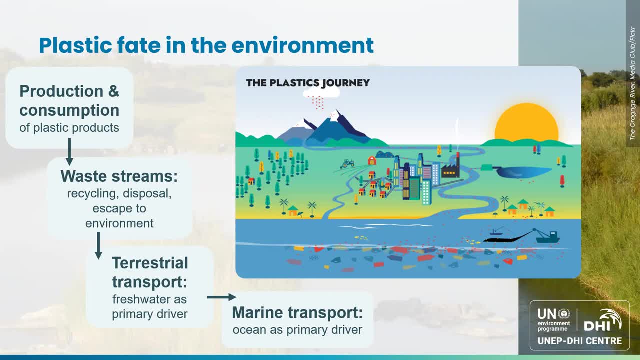 The issue of plastic pollution requires a comprehensive set of data and information that covers the whole process, And this includes the whole life cycle of plastic: when plastic has been produced, when it is consumed to the point where it's being disposed, for example, landfill, or it's being recycled. 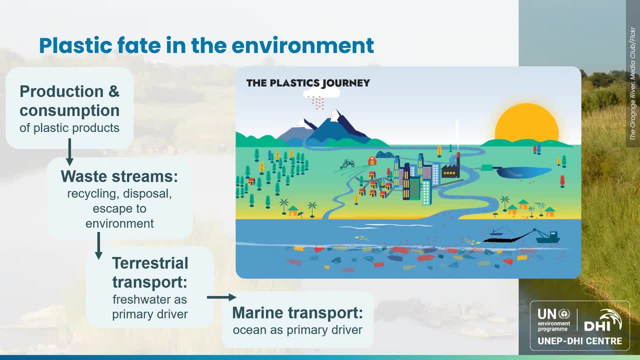 and then, eventually, how it reaches the environment, becoming part of plastic pollution, through the inland, from the freshwater ecosystems and then, eventually, when it reaches the marine ecosystem. So, as you can see, in this plastic journey there is really the need of you know. 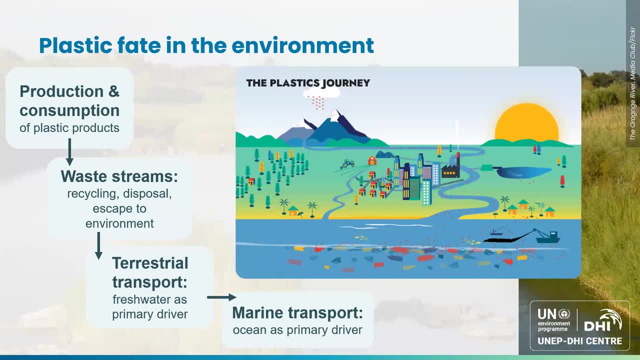 different type of data sets, different type of information that goes across different themes and often different, let's say, organizations or institutions that are maybe not always talking in the same way. They're not maybe always talking together, And this is where, of course, the need of coordination. 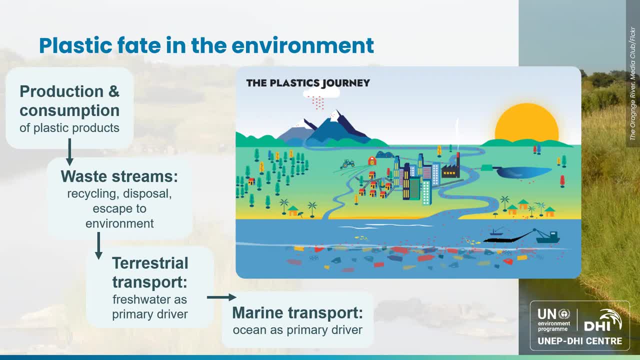 and harmonization of both the way we talk about plastic, but also the way these data are being collected and made available, is fundamental, And Carla highlighted this already is one of the tracks that the GPML is focusing on is harmonization, is community of practice. 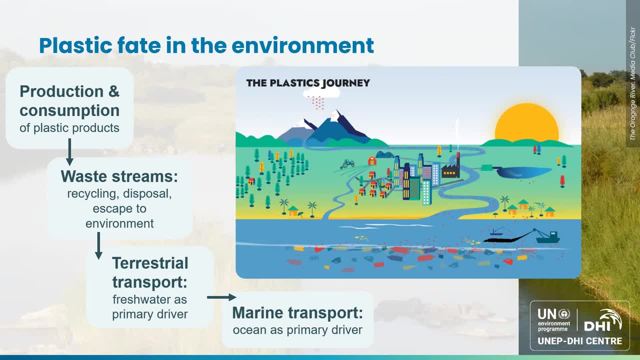 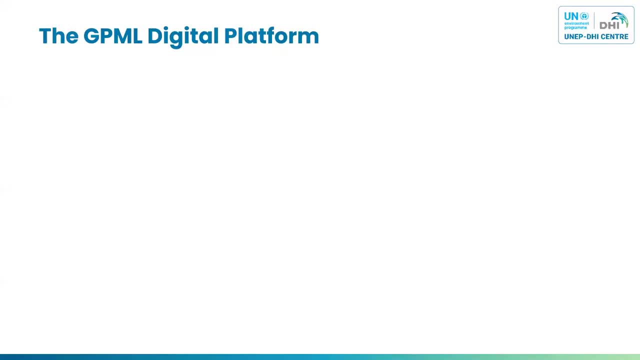 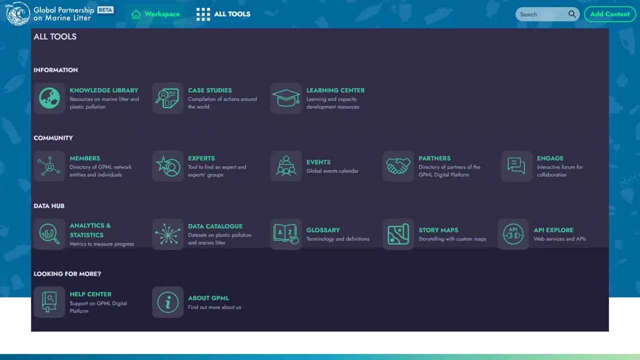 is really dialogue across stakeholders, And this is also one of the key activities DHI, or UNM, DHI has been involved with. And if we could go to the next slide and apologize for these animations, please click a couple of times. What I want to make aware you here is that all this information- 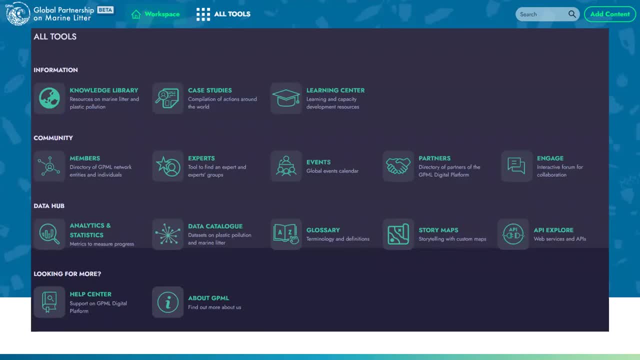 all these tools are made available through the GPML DIGITAL platform, which is really the place where many of the work that UNM DHI is doing and GPML and UNM is doing is accessible. So it's really key resource And what you can see here. 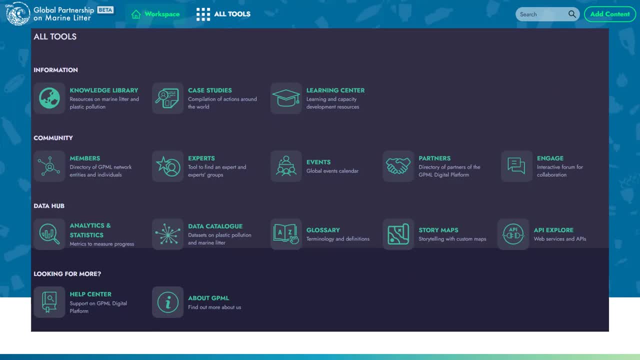 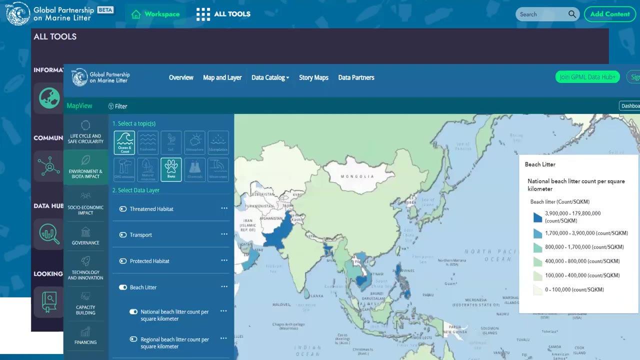 there's a set of different tools and locations where you can access information and data that can help you when planning and implementing intervention to address plastic pollution. And, if you can click one time more, one of the tools I would like to highlight is the Data Hub. 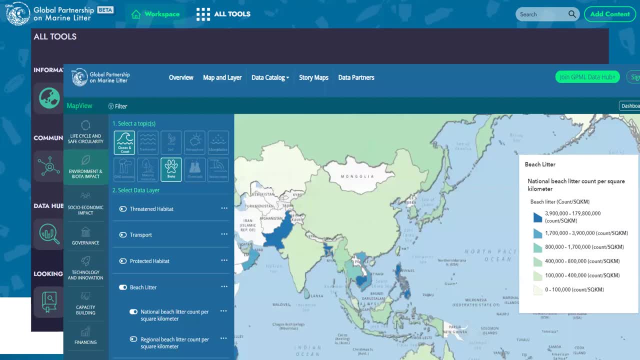 because this is really the location where the, as Carla said before, there are more than 300 data sets that are available through the platform. The harmonization process will allow to make this data available in a harmonized way through the Data Hub, which is the application that you can see here. 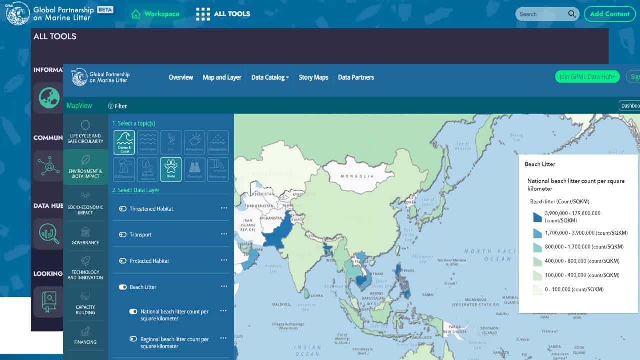 through a set of right now is more than 100 indicators which are based on this harmonized data set. What I would like to highlight- last thing before we move to the next slide- is that if you look on the left here, what you can see is that there is different way of like this. 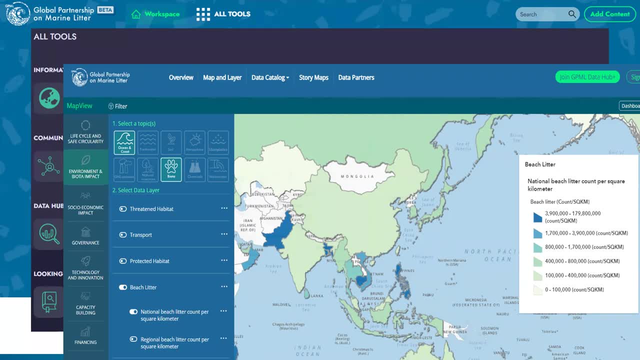 these indicators are being grouped, And what I want to highlight is that there is not only information around plastic life cycle or plastic in the environment, but, as I mentioned before, it is important to look at other aspects in order to make effective intervention And for this reason, 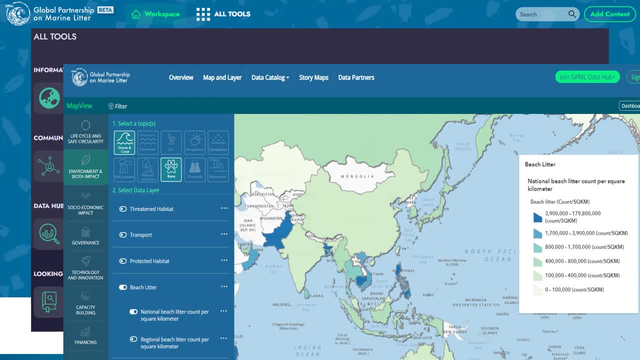 we look at harmonizing and making available also different type of data set, like, for example, around socioeconomic impact, governments, governance policies, technology and innovation financing, knowledge sharing. So we really try to look at the issue in a broad way. 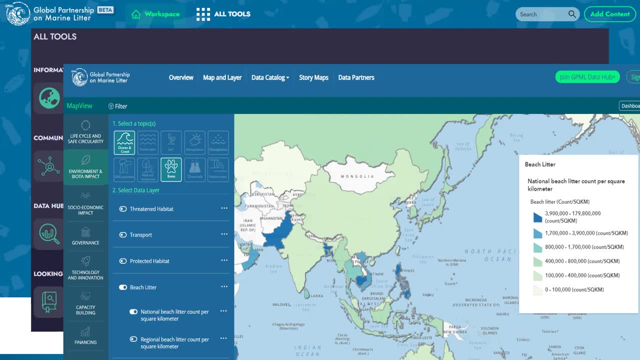 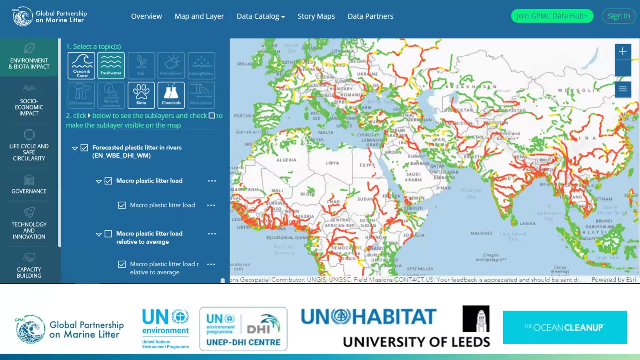 and make all the information, all the needed information, available. I would like to bring an example of one of these data set And, if you could go to the next slide, this is the one that I believe Heidi already mentioned in her introduction. So one of the first thing we've been looking at is: 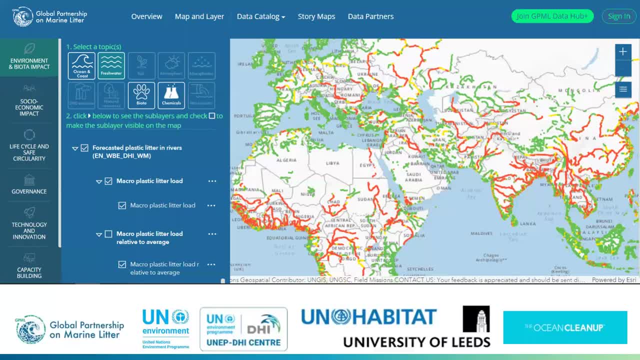 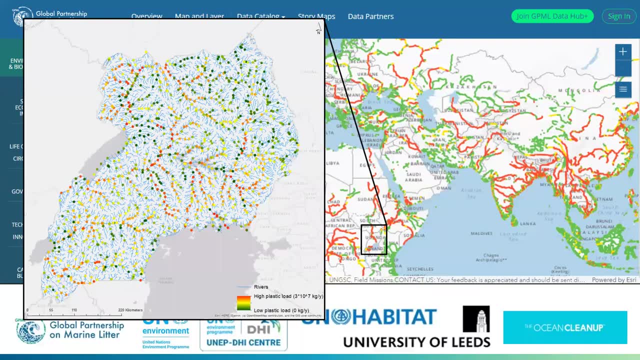 from UNFDHI side has been to try to map or estimate a plastic leader in rivers, And this is because many are aware of the issue in the marine side but not everyone is aware or there's not maybe the same emphasis on the issue of plastic pollution in freshwater ecosystems. 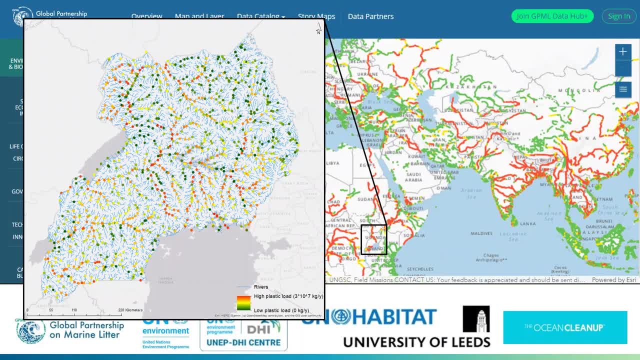 So the first thing we did with several partners like UNHabitat, Ocean Cleanup, University of Leeds, UNEP, GPML- we tried to estimate and evaluate what is the plastic concentration in all rivers around the world And in the close up here. 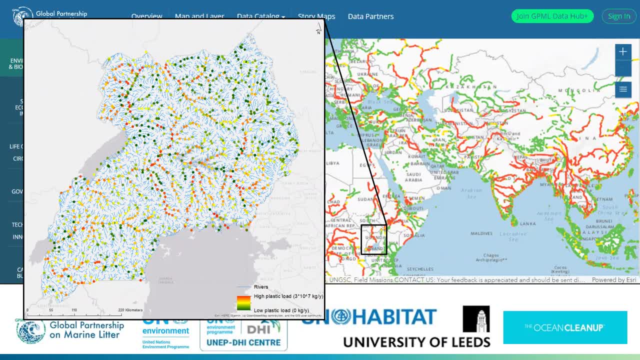 you can see an example of how can this data set, how this information can be used at a national level. So what you can see here is a country- Uganda- where you can see the data set allowed to map and understand in a consistent way. 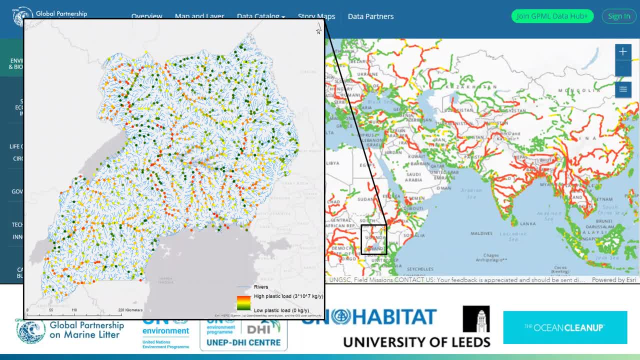 what are the concentration of plastic pollution across the rivers in the country? And then this, of course, is helps in understanding the Asian freshwater ecosystem, but also can be put next to information around where plastic has been generated- industrial sites, landfills- and really trying to understand. 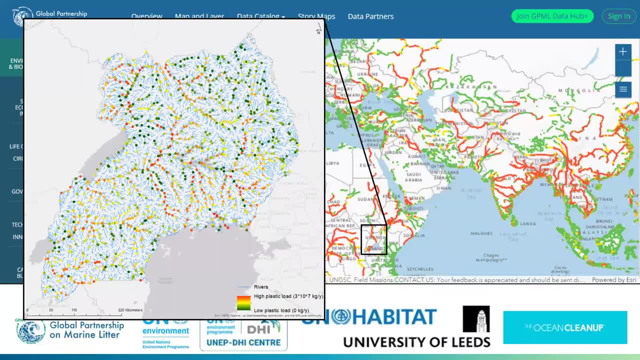 you know where the issue originates and what are the most effective intervention. We're actually in the phase now of testing the opportunity to do some kind of scenarios both with GPML and also with the Ocean Cleanup in order to inform their activities. If you could go to the next slide? 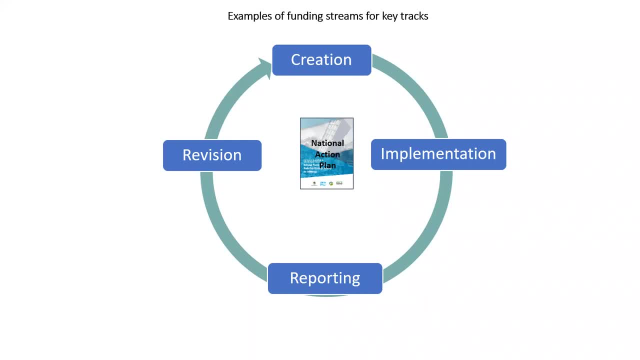 as I mentioned earlier, I also wanted to a little bit. so there is a lot of data needs, as I've highlighted, but of course this requires funding, this requires support from this organization, And here we have collected a few ideas around how we see. 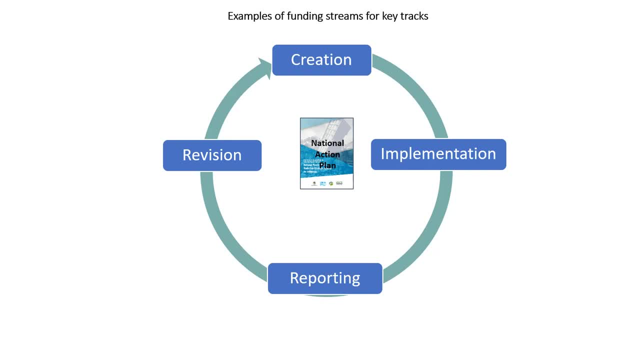 you know which partners are required and how we see funding opportunities to be. you know how can different funding opportunities come in in order to tap into the process. And if you could click a few times, there are a few. sorry, there's an animation here again. 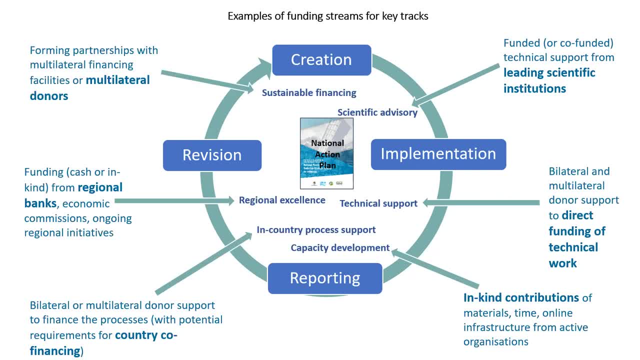 I love them. But so the first thing I want to emphasize is that during the early phase, during the creation, implementation and also reporting, there are some key aspects. that involves scientific advisory, technical support and capacity development. All these requires input from 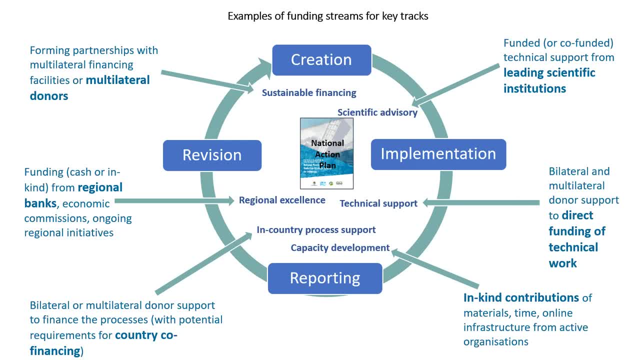 you know, scientific institutions And there are different ways. this, of course, can be quite a costly process, but there are different ways where we see that there is support that can be done through the process. This is both through, for example, bilateral, multilateral donor support. 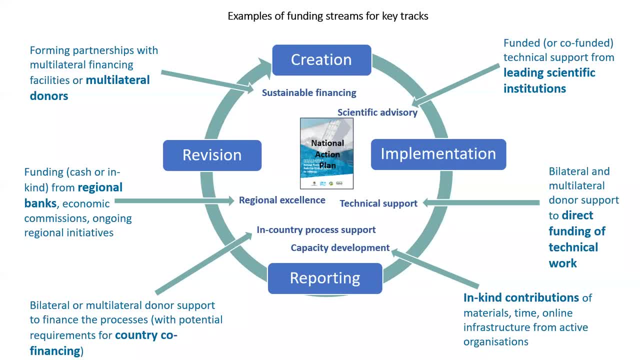 as well as, for example, connecting to leading scientific institutions that are already active in the field and can provide co-funded support in the implementation or the development of action plans. If we look at the second half of the slide, so more on the left side, 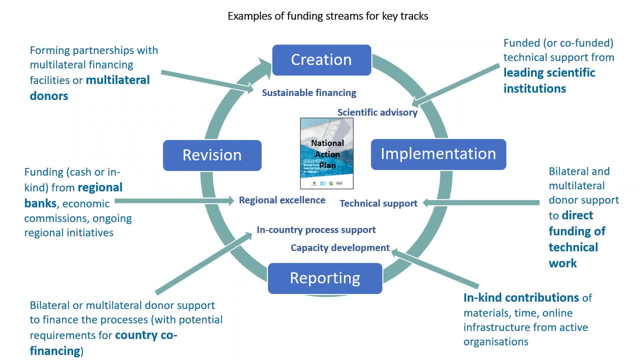 there are, of course, key aspects here also requiring you know, for example, connection with the regional excellence, so ensuring coordination at the regional level, And here there are several regional bodies, regional banks, regional initiatives that can be connected to in order to provide support. 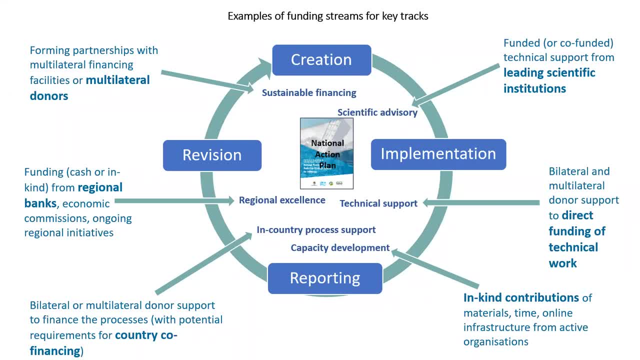 at this step of the process. And finally, one thing I would like to highlight, maybe slightly leading into the next presentation, is that, of course, there are several partnership and multilateral donors that are providing support for this kind of process. One thing we hear: 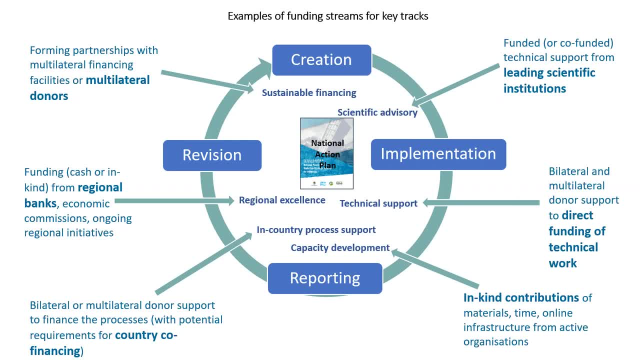 we often hear and we believe is also really important in order to ensure sustainability of the development implementation of the action planning over time is, of course, that the countries where the action plan is being developed is fully on board and is driving some of the in-country process. 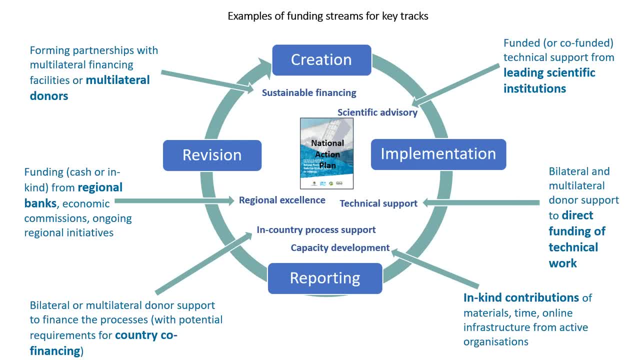 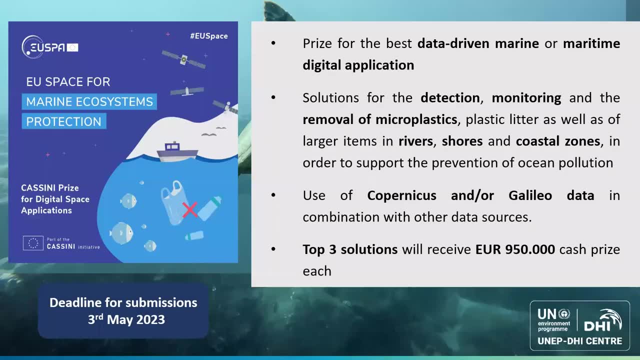 through also some co-financing And, as this last slide just to say thank you. I also want to highlight the opportunity that there is for the Cassini Prize. This is a prize by the European Union where there is, which will award the three most novel digital application. 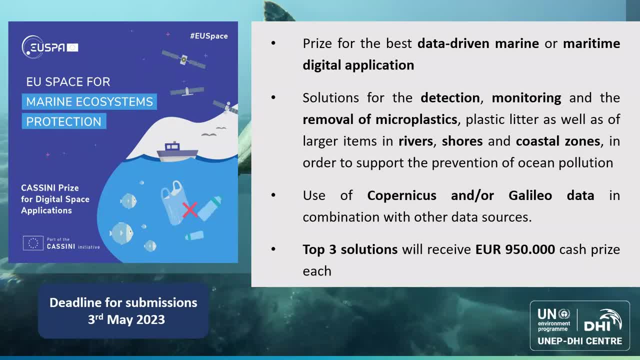 based on Copernicus or Galileo data in order to monitor or remove microplastic. And I just want to highlight this- The deadline is the 3rd of May, so there's still a bit of time, So hurry up for any of you. 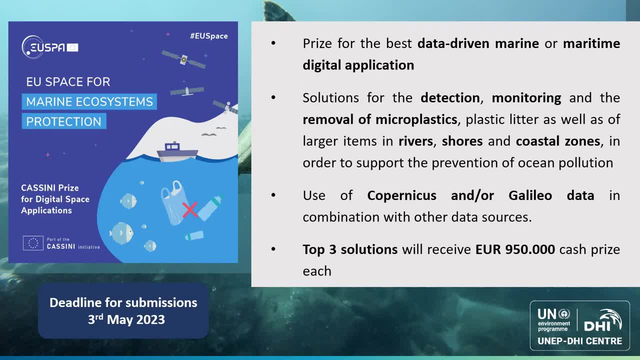 that is interested. Thank you very much. Thank you, Nicola. Excellent presentation and an excellent ending, And this is great for people who are interested and perhaps already active within the data domain. Just wanted to remember to all the participants. I saw we already received some questions. 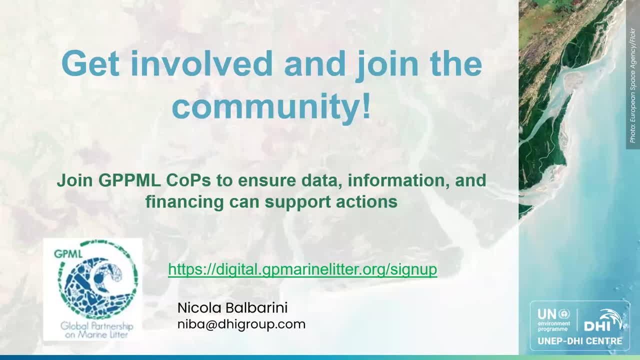 in the Q&A and chat section. Please feel free to add those as we go along the presentations. We'll make sure to pick those up in our Q&A slot after the third presentation. So thank you, Nicola, for your presentation on the data side. 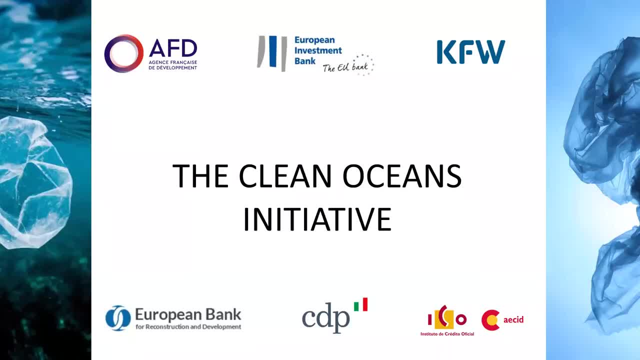 With that we have our third presentation of the webinar. We're really happy to be joined by Juan Bofill. Juan is senior water engineer at the Water Management Division at the European Investment Bank. Juan holds master's of science degree in civil engineering. 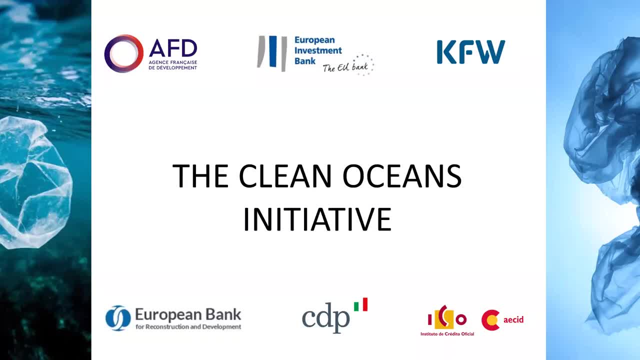 and is currently senior water engineer at the EIB. as I mentioned, He's also responsible for the water sector portfolio in Latin America and Caribbean. During his 25 plus years of professional experience with the private and the public sector, Juan has been responsible. 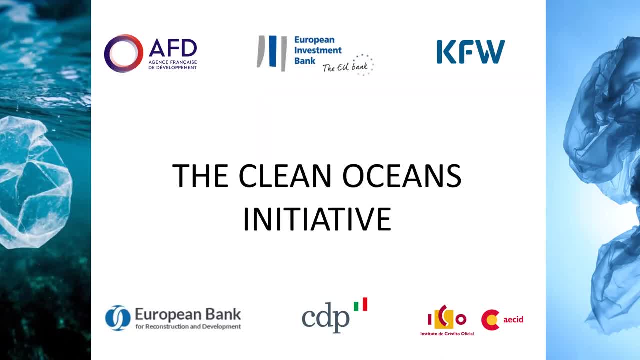 for business development and project management, both within the broader water and wastewater sectors Within EIB. he's also managing the Clean Oceans Initiative, And that initiative we'll be able to learn a bit more about today. With that, Juan, the floor is yours. 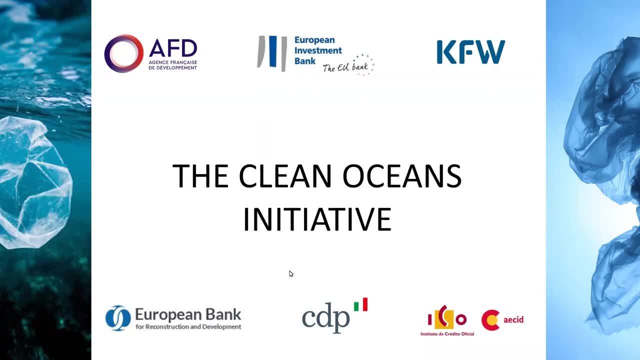 Thank you. Thank you very much, Maya. It's a pleasure to be here in this webinar, Also with this previous presentation, which are really really interesting. I'm very connected to the Clean Oceans Initiative. Thank you, DHI and UNEP. 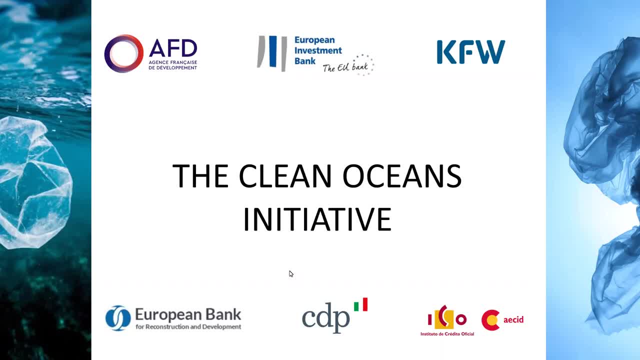 for inviting me Today. I'm representing a group of financiers at the end in this Clean Oceans Initiative. As Maya said, I'm working in the European Investment Bank. For those who do not know the EIB, we are the EU bank. 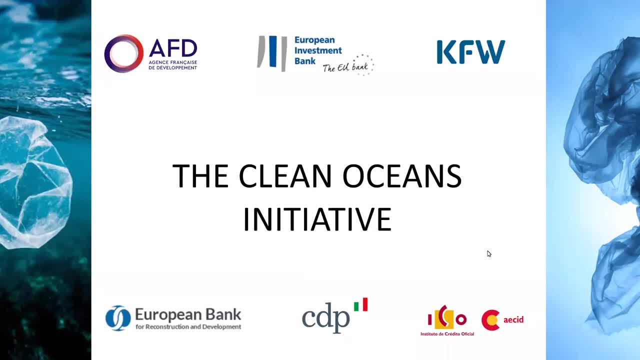 I mean, the shareholders are the 27 members of the EU And what we do is we finance projects inside the EU and outside the EU. But basically what we do is we finance every year approximately 65,, 60 to 70 billion euros. 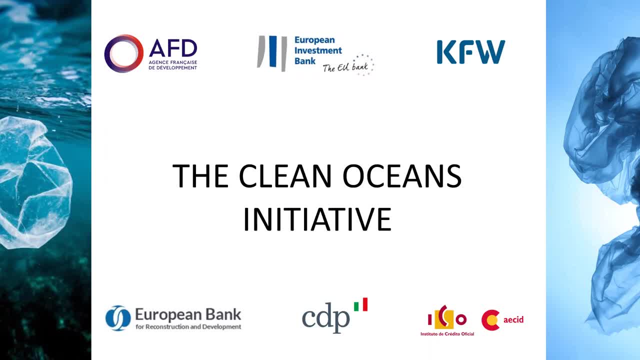 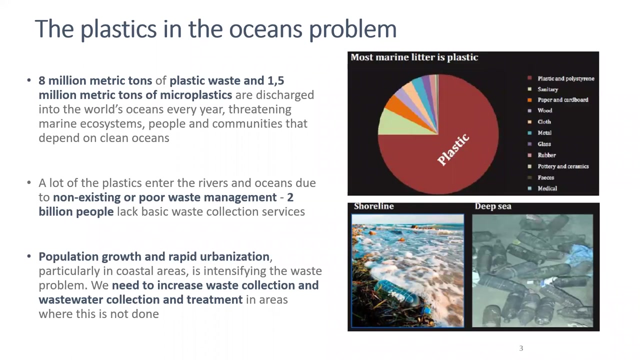 in projects, And some of these projects are targeting the ocean health. So some time ago we decided to create this and I will try to explain it in this presentation, Next slide, please. Okay, so everybody was mentioned before and everybody knows this. 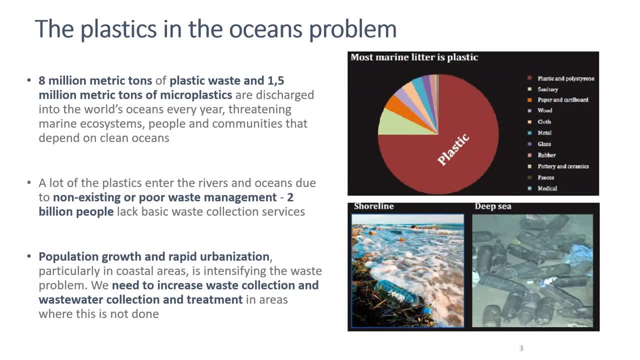 the issue of plastics in the ocean. We hear a lot, these 8 million metric tons of plastic waste that is being discharged every year into the oceans, But at the end of the day, it's much more Recent studies and we can hear that we're talking about more. 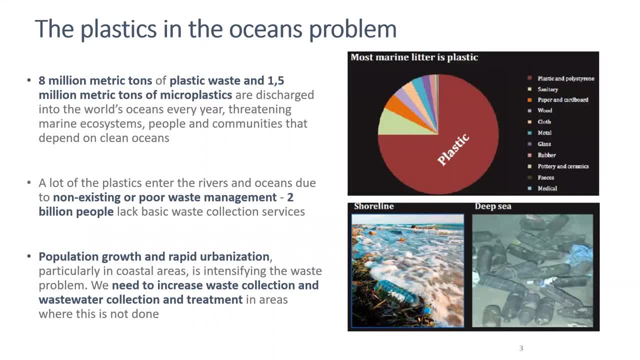 We're talking about 12 million metric tons, And this is because, besides of the 8 million of mismanaged plastic in the coastal areas- because this 8 million was calculated with a study only considering coastal areas- we have also to add the 1.5 million metric tons. 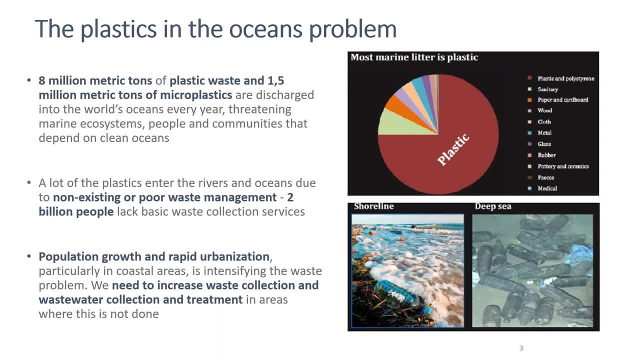 of microplastics. that was already mentioned before. But besides this 1.5, we have also 0.6 metric tons per year that is discharged directly from sources at sea, For example fishing nets, Or also we have to add 2 million tons. 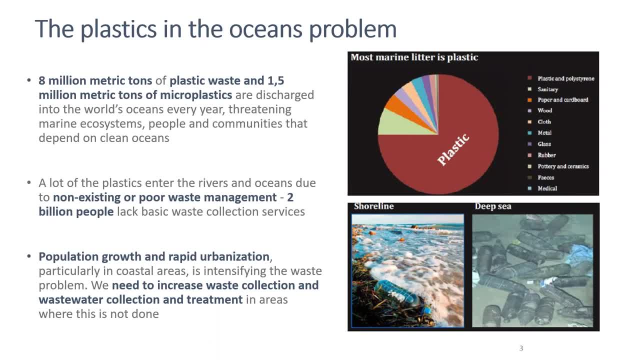 that are coming from inland. This is also connected with Nicolas, because he mentioned, a lot of plastic is discharged through water, lands or rivers, not only in the coast. So this is impact. I mean the main issue, one of the main issues here. 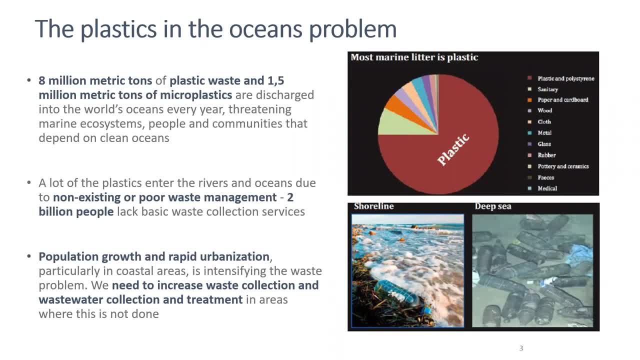 is that there's not or is a poor waste management in the world. in many regions, It's calculated that at least 2 billion people lack of basic waste collection services, And this ends up in the rivers and the creeks and, at the end, into the oceans. 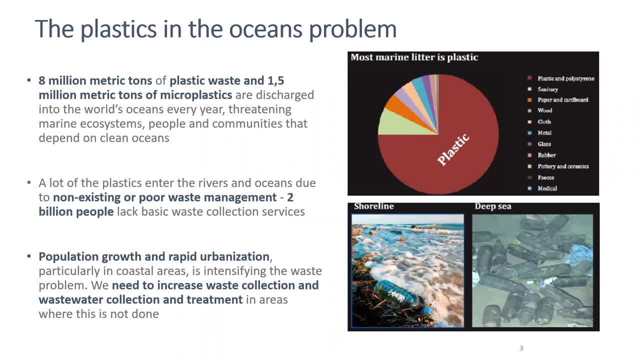 In the same way, the population is growing and there's a rapid urbanization And in all, particularly also in coastal areas, a lot of people lives in the coast. So another issue that is happening is that many of these coast coastal countries. 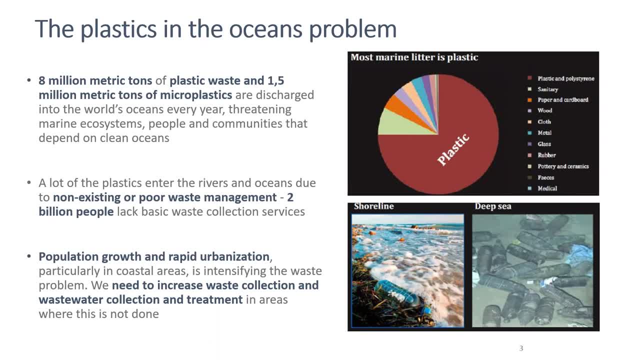 and coastal populations do not have a wastewater collection, for example, And this is has a huge, has a huge impact into microplastics. Can you, can you next slide, please? Okay, So this comes from another tool and not exactly the one. 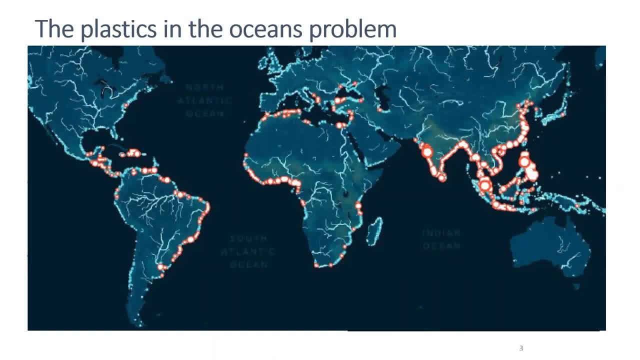 that Nicolas presented, which is also quite interesting. So this is not a competition of who is showing the nicest tool for evaluating the plastic discharge, But this comes from from, from another digital platform that shows, shows how, every moment, if you click in. 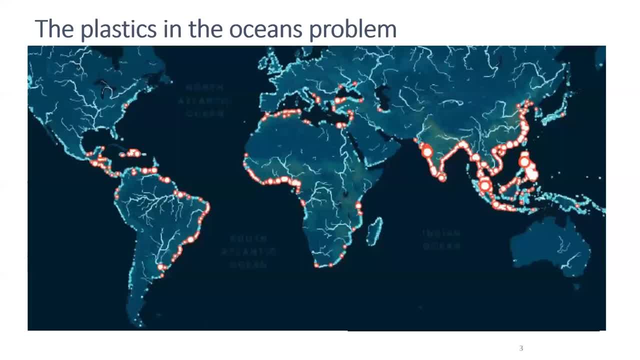 in that particular point or particular dot, you will see how much plastic is discharged in into the, into the, into the ocean, through this river, And, as you can see in this, in this snip that I took from from from there. 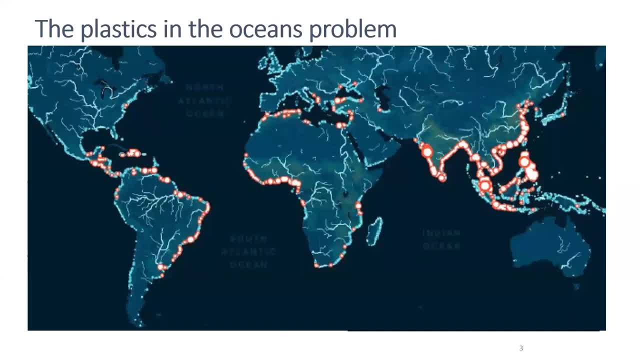 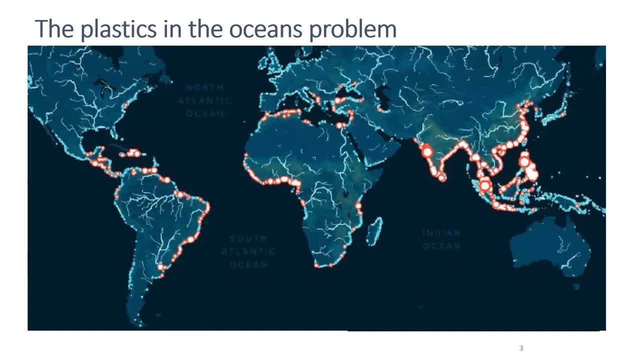 the, the, the country itself. Of course, if you Zoom you, you can you can notice that, But it's true that the main problem is in many regions in the world, But of course Asia and Pacific is one of them. 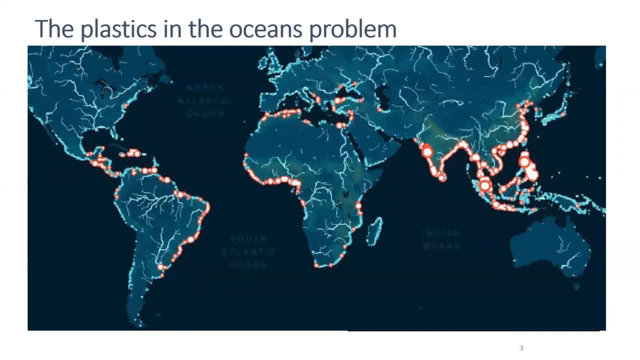 Other other regions are, of course, Sub Saharan Africa, where the there's no plastic solid solid waste, And also in Latin America. In Europe we have this problem, but it's of course. the solid waste management has been improved significantly since all the countries joined into the EU. 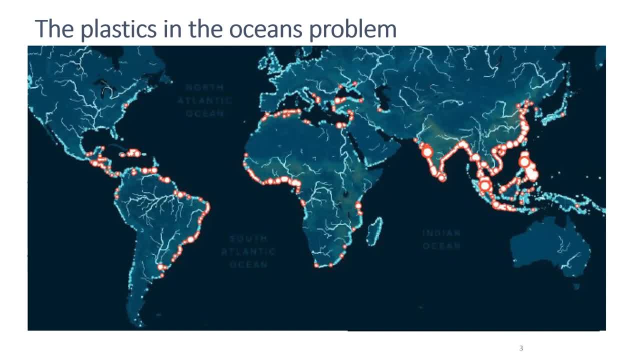 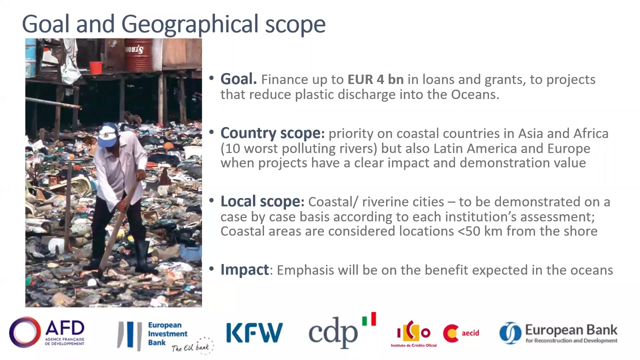 But we can also find issues, of course, in Romania and Bulgaria, in the Black Sea, So the problem is global, as you can see. Next slide. please, Just facing some kind of delay in the slide. OK, thanks. So what's the goal? the COI, These institutions that you have below in the slide, AFD, which is the French Institution, Development Bank. 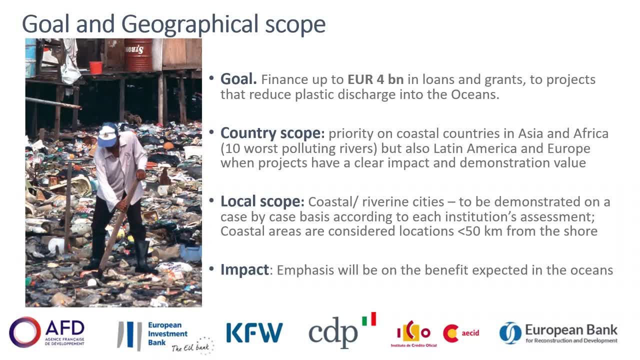 ourselves: KFW, which is the German Development Bank, CDP, which is the Italian Development Bank, Ecoacid, which is the Spanish agencies for development, also in the development banks, something similar institutions. And the European Bank for Reconstruction and Development, the EBRD. 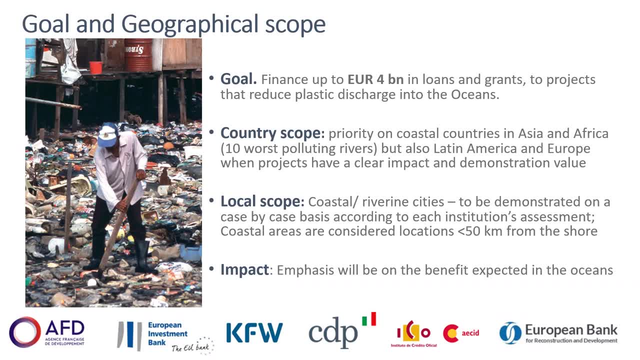 We all decided to have this kind of facility in order to finance up to four billion euros in laws and grants to produce that reduce So projects that have an impact in plastic discharge into the oceans. Four billion is a lot because we can consider that, for example, the EIB can only finance 50 percent of a project. 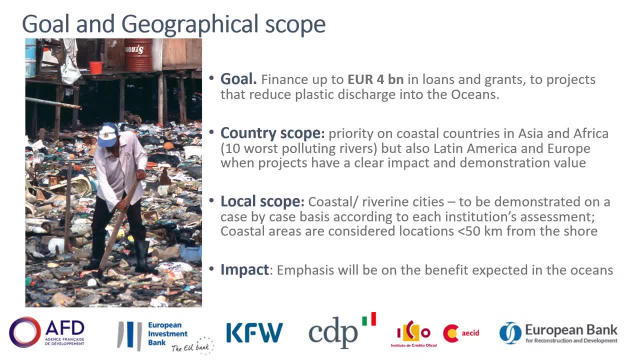 So we are talking of at least more than eight billion euros At the end of project costs, total project costs, but our financing is up to four billion. So the country scope- as I showed before in the slide, it's mainly should be Asia and Africa. 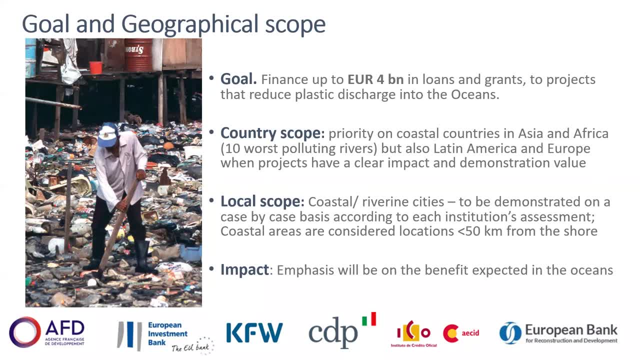 So because these countries, these continents, have the 10 worst polluting rivers, but also Latin America and Europe. when we can show that the projects have a clear impact in the reduction of plastic, it can also be eligible or labeled as Clean Oceans Initiative. 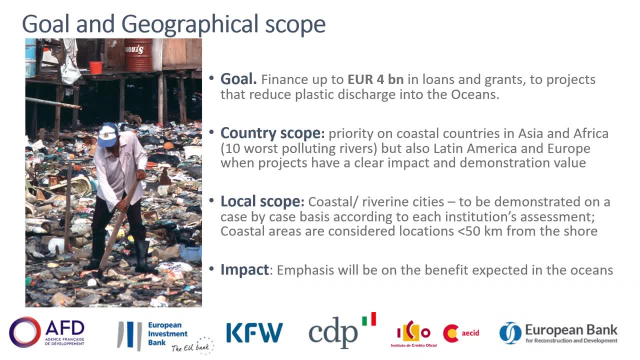 We also consider besides of the 50 kilometers, because for us and for the EU, 50 kilometers is considered coast. The distance of 50 kilometers to the shore is considered coast, But nevertheless, in special cases, when we have rivers that are really significant and there's no solid waste in these rivers, 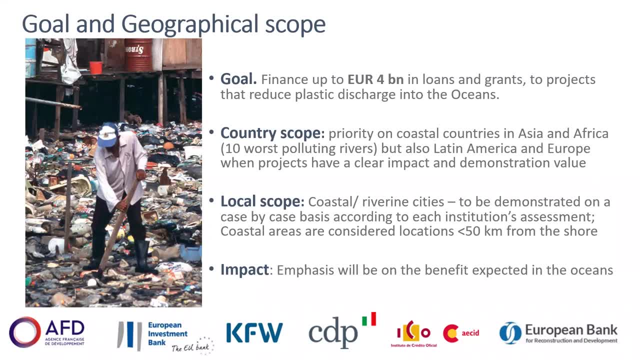 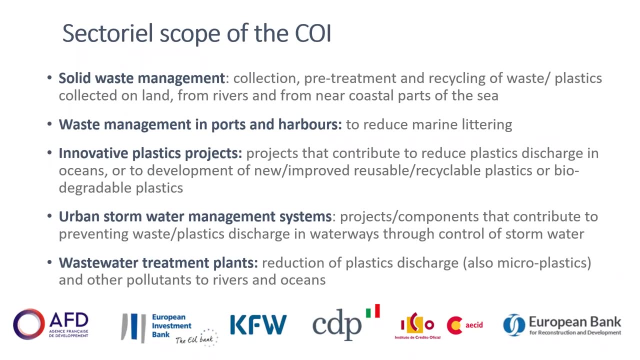 we can also consider this as Clean Oceans Initiative, because, at the end of the day, this pollution gets into the oceans as well. Next slide, please, Okay. so what do we finance with this four billion? The idea is to finance solid waste management. 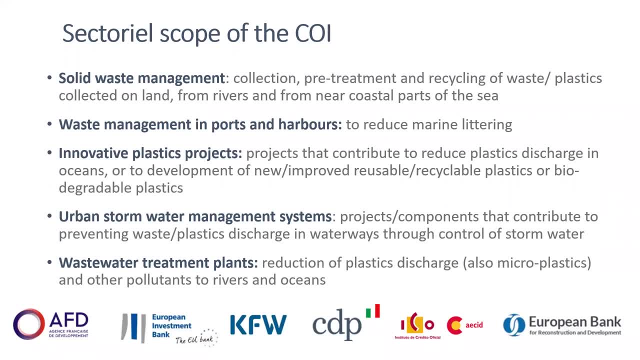 We, as I explained before, with a solid waste management, we cannot proper solid waste management. we cannot address this because, as you can see, it's important to mention this. We are talking about end of the pipe solutions all the time. 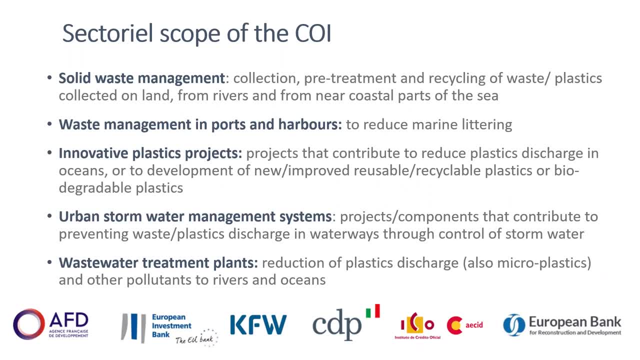 We are not addressing. we are trying to finance projects in order to solve the problem when the problem has already been created. We rely on other institutions as well And we will see in the future if we have the capacity to also to change the policies in the countries. 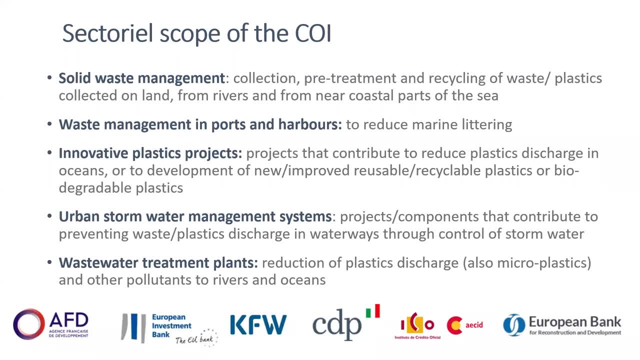 in order to that plastic does not end in the solid waste- let's say sector at that time- but in the solid waste cycle. But initially, at this point in time, what we are doing, trying to address the problem as it is now. 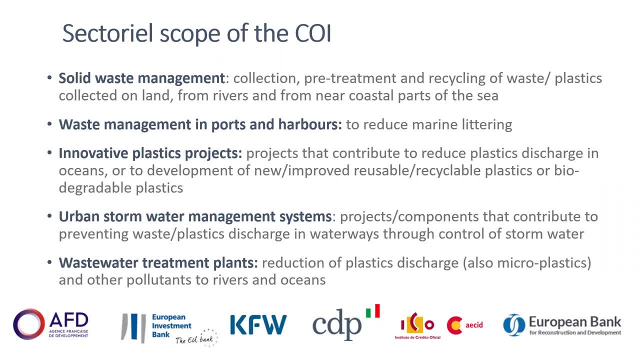 So solid waste management projects is something that we are targeting. We are targeting as well solid waste management in ports, because it's directly related to the ocean, So the immediate effect will happen. Also, innovation in plastic projects. So plastic projects that can improve the reusability or recyclability of plastics. 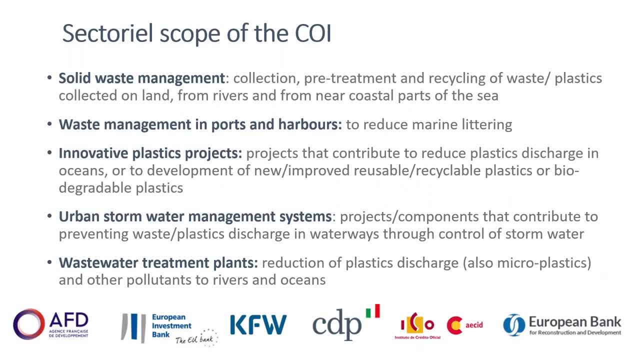 It's also something that we're targeting- And, of course, the water sector, because the water sector is quite relevant in two ways. One of them is the urban stormwater management systems. We always see when we have open creeks, for example, open drains. 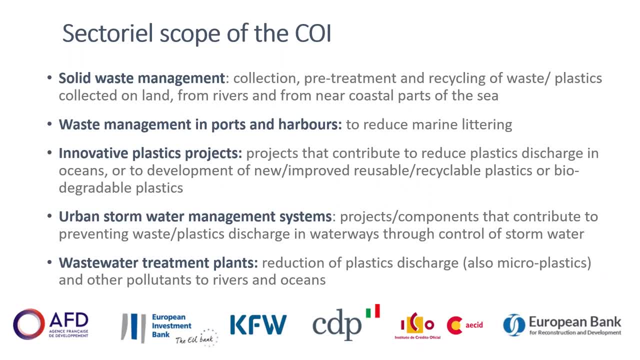 they discharge, they are basically landfills of plastic. So then, when the rain comes, everything goes into the river and into the oceans, And also collection and treatment of wastewater, because it has been proved that at least with conventional wastewater treatment plants, we can reduce up to 90%. 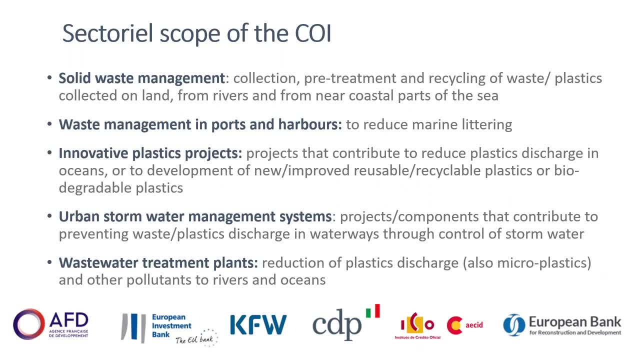 Of the microplastics that enters into the wastewater. The issue we have here- and it's something that we need to solve- is that the microplastics end up into the sewage sludge, And so we are always looking for solutions internally in the COI. 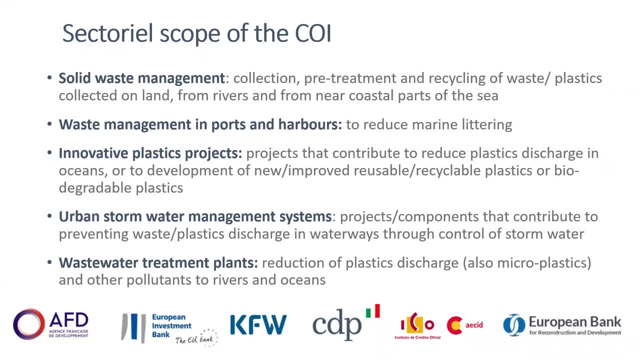 looking for solutions with pilots trying to find pilot plans to reduce that, to reduce the microplastics discharge into the solid waste- Sorry, into the sewage sludge. Because then if you reuse the sewage sludge for, for example, as a fertilizer, 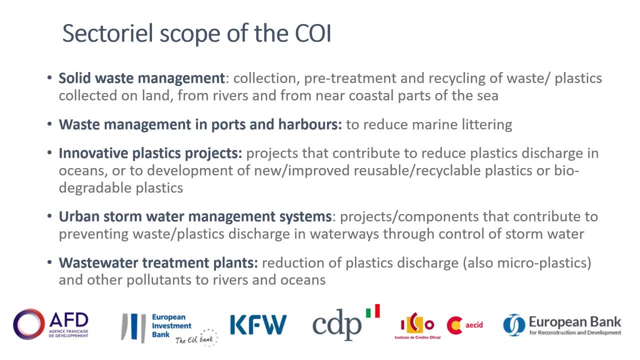 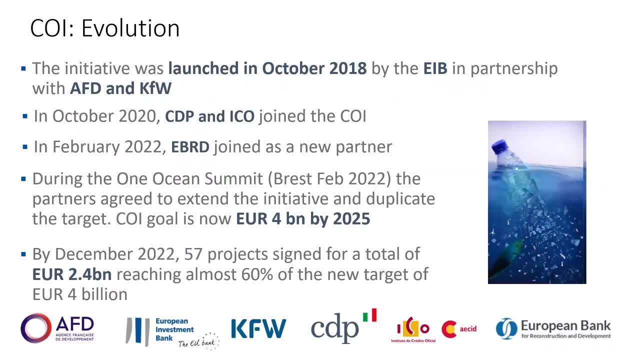 then the microplastics come back into the system. Next slide, please. So basically, this is where we are now. Just to mention that the initiative was launched in 2018.. So it's something that is not really new. Initially, we were only EIB, EFT and KFW. 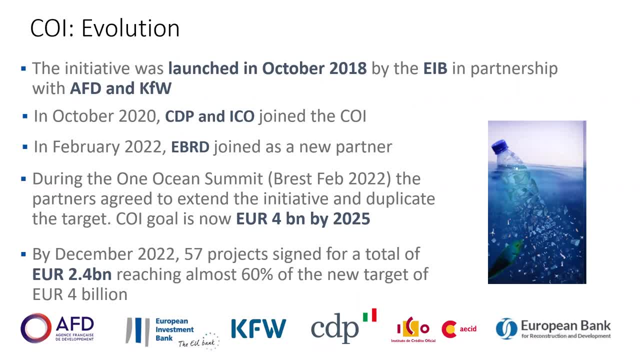 But all the colleagues that I mentioned before, many of the other institutions, joined during this time And when we saw in February 2022 that we had already reached almost 2 billion euro, which was the original target, we decided to extend it, to extend it up to 4 billion. 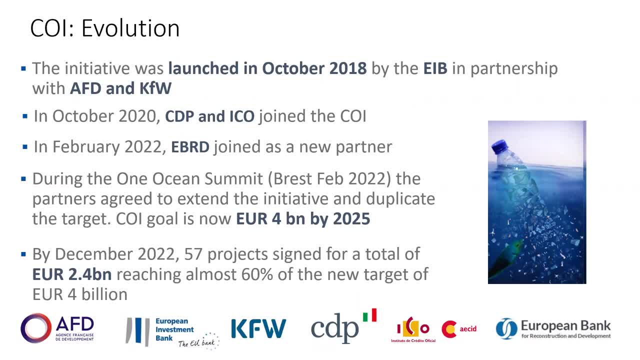 And also to extend it and also to extend also the deadline. So instead of 2023, December 2023, it will be December 2025.. So we can see that every every three months that we get together, we incorporate more projects. 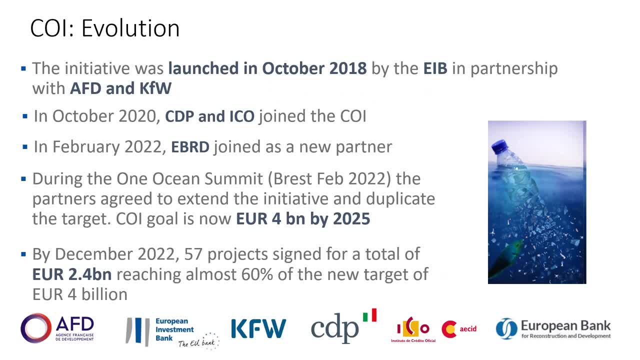 Right now we are at 2.4 billion on almost 60% of the target, which is quite, quite remarkable: 57 projects. It's what we are assigned as the Clean Oceans Initiative And my last slide, Thank you. 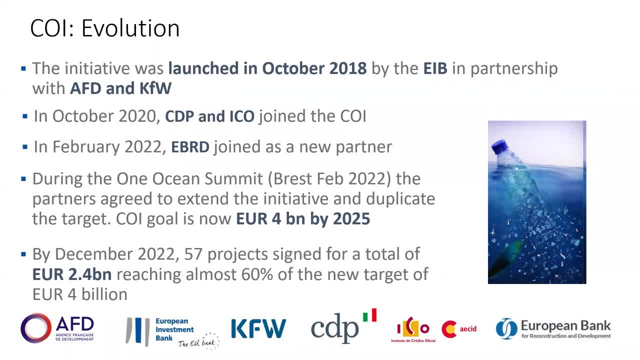 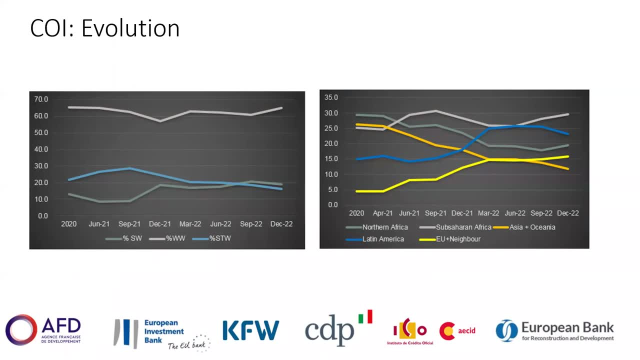 Can you please move to the next one? I know sorry, it's not this, It's another slide. This is the evolution of the Clean Oceans Initiative. What we saw is that, out of the 57 projects, what we have is that 20% is solid waste projects. 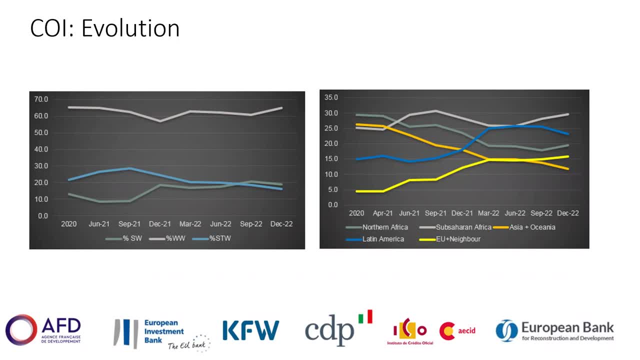 So we are looking for a solid waste project. We have facilities for that, trying to identify them, But currently what we're having is a lot of wastewater projects, which is also quite eligible for us, But indeed the solid waste is underrepresented. 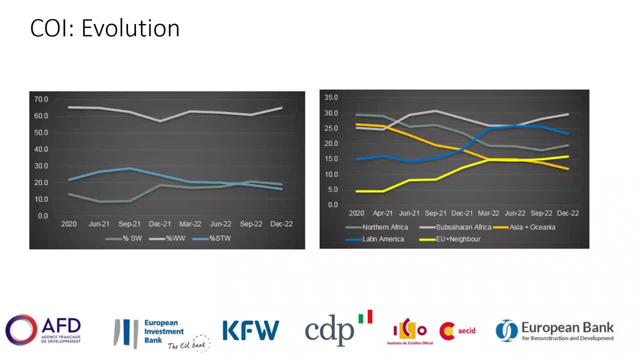 So we are looking for that in order to improve that And in terms of on the right picture, you see where the projects are located, And most of the projects are in Sub-Saharan Africa and in Latin America. Some of them are in Asia. 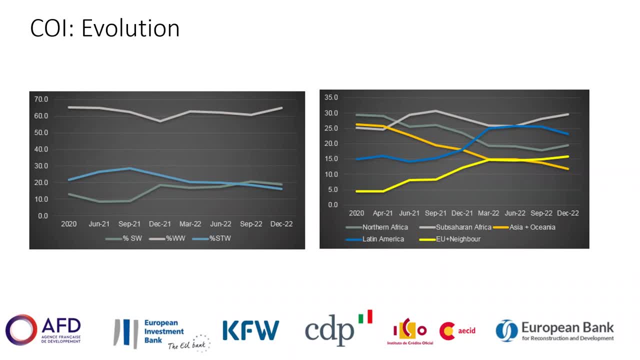 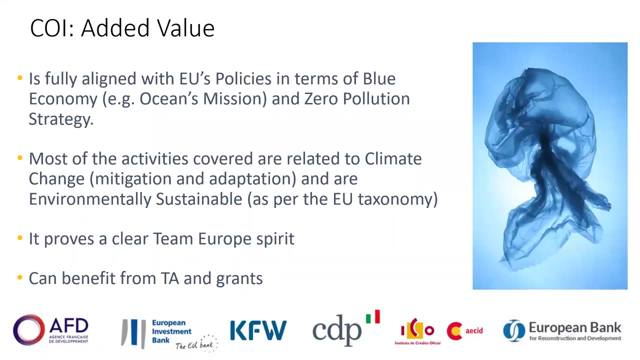 So Asia, in this case, is underrepresented: Asia, Oceania. So we are also looking for that. Try to solve that, Try to find more projects in these regions. And last slide, Next slide, please. Okay, So the point for us is that the Clean Ocean Initiative. 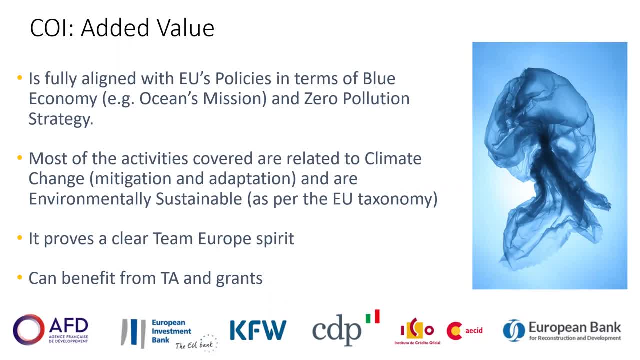 is fully aligned with the EU policy. The EU has a very sound strategy for blue economy, For example, emissions- It's called ocean emissions- So we consider that as very fully aligned- And also with the zero pollution strategy that was launched in May 2022.. 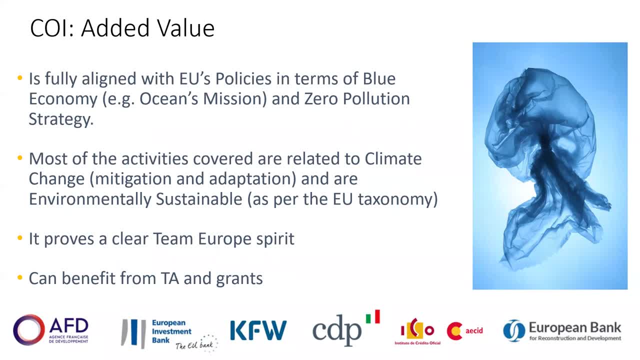 So most of the activities covered by the COI, by the Clean Ocean Initiative, we have seen that it's also linked to climate change in terms of mitigation- for example, for the wastewater treatment and the soil waste- and adaptation in terms of, for example, 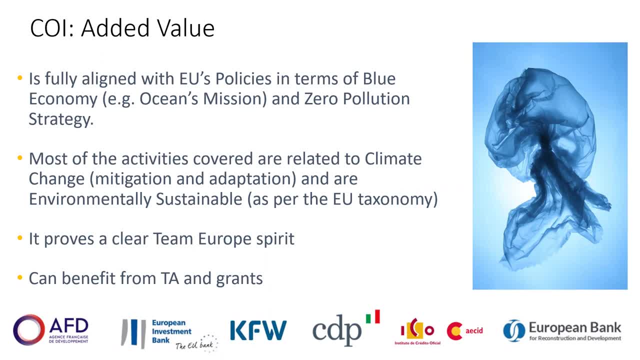 the stormwater management And are what we call environmentally sustainable. We are at the EIB as the EU bank. we are working with the EU taxonomy. It's another topic that we can discuss another time, But we are aligning with the taxonomy. 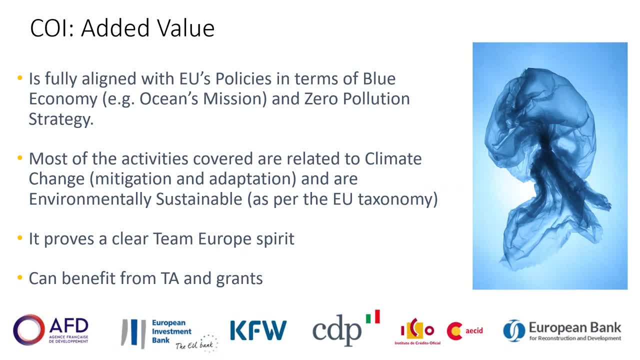 And the activities included in the COI are, in general, aligned with the EU taxonomy. All the institutions that you can see below are European institutions working abroad, working outside the EU, So inside the EU and outside the EU. So what it proves is that we can associate. 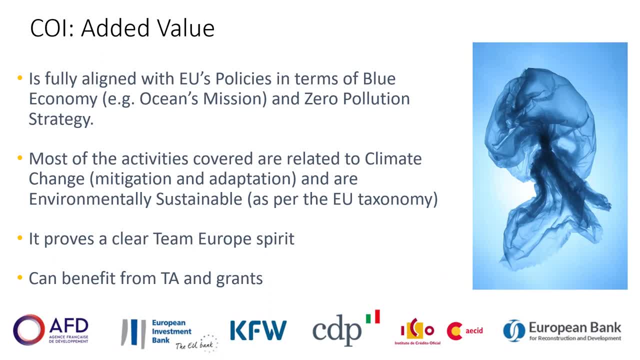 all of us in order to fulfil this common target And it's important that this in the future- and we are looking for the way to do it. these projects can benefit from technical assistance for preparation and implementation and also grants one part of the grant. 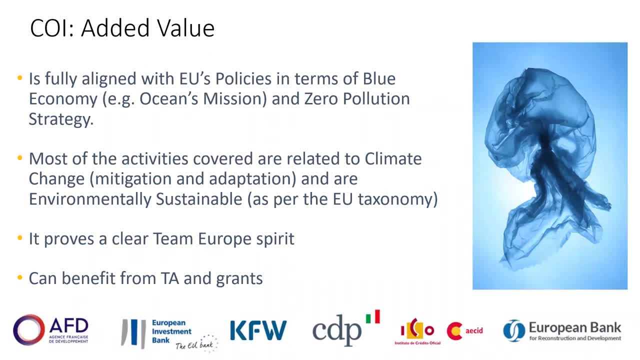 We see that a component is specifically, very well, very targeting what we are looking for. Why not? We can try to channel a grant. So thank you very much. That was my last slide And well, there's another one Thanking and with some links. 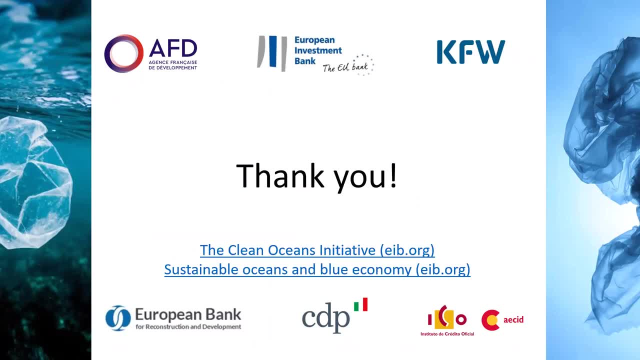 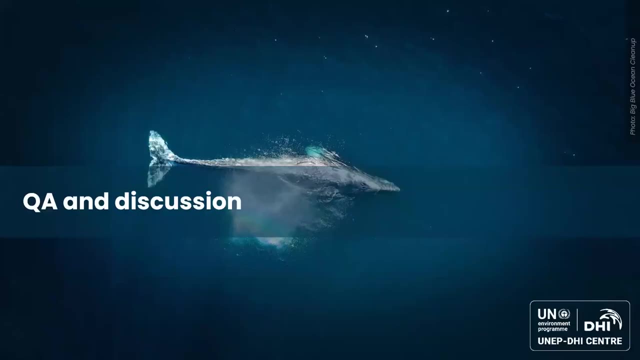 So, thank you, Happy to discuss any question. This is excellent. Thank you so much, Juan, for the presentation, And thank you to all the presenters who prepared PowerPoints for today. I think it was a really great introduction to the overall picture and the background. 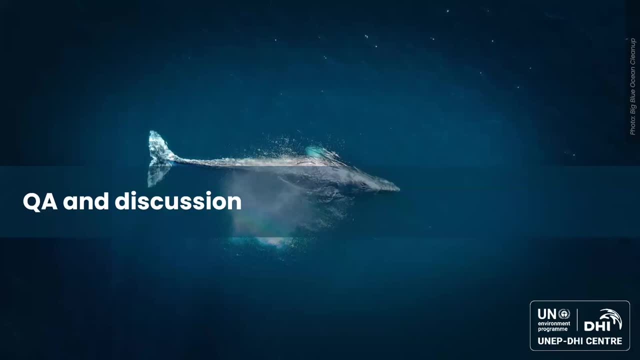 we have for these activities, diving into the data, the partnerships and the financing part. So we're covering all the sort of aspects that are needed for real action on marine litter and plastic pollution. With that we have approached the discussion session. We already have few questions here from participants. 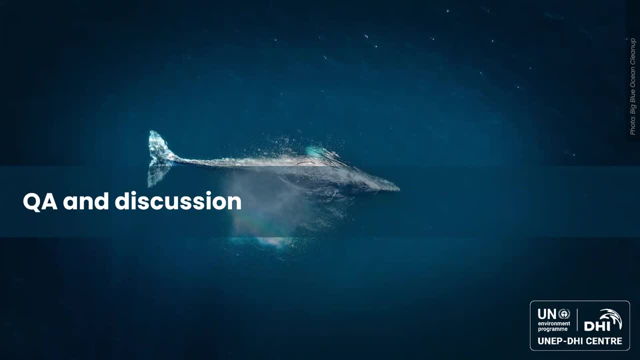 But again, I encourage you to write your questions either in the Q&A box or the chat, And we do have some time to answer them, So go through these now. To kick off, I would like to turn back to you, Heidi. 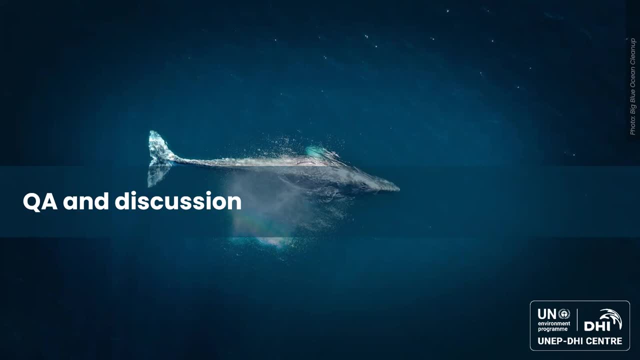 since you gave a great introduction of the overall and policy and international background for these activities. So I have a question for you if you would be able to unmute your mic and give your perspectives. You mentioned the national action planning processes And of course, here we're talking about data. 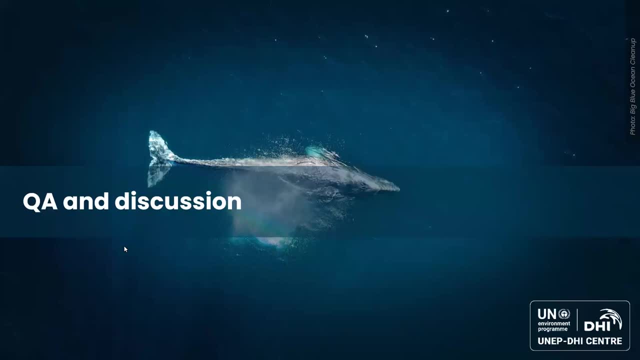 about very concrete actions. I wanted you to give us your reflection on the national action planning process and how do you think that has worked and has the potential to work to help identify these locations or specific projects and actions for intervention, If you have any examples from previous national 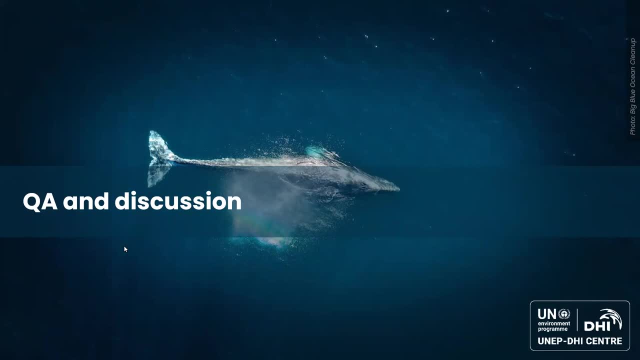 and regional action planning processes or the forwards look. I think that would be great to hear from you, Thanks. Thank you so much for that question And yes, we've been working on action plans for quite some time. First we started on regional action plans. 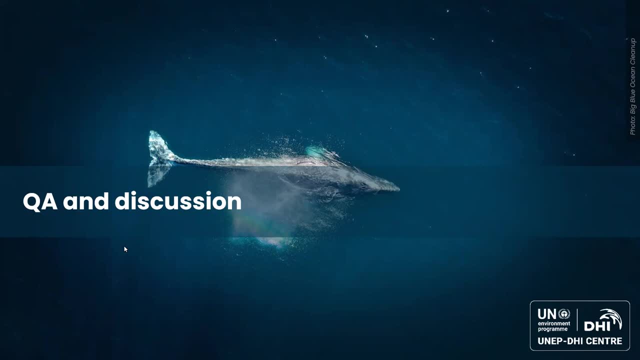 and that's been really around zooming in on the problem in regions, And I do think that those type of processes help stakeholders and governments to consider the aspects on plastic pollution and marine litter And I think it has led us to elevate the issue from 2008,- 2007, when we started working. 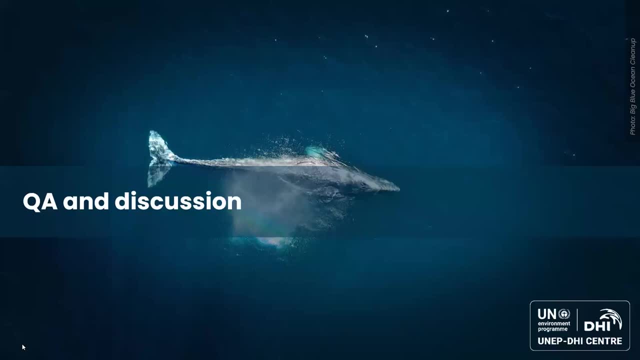 on regional action plans to today, when we are focusing more on national level action. So the way we've approached the action plan process is to look at how do you identify what type of data and information you already have? Who are your stakeholders that are operating? 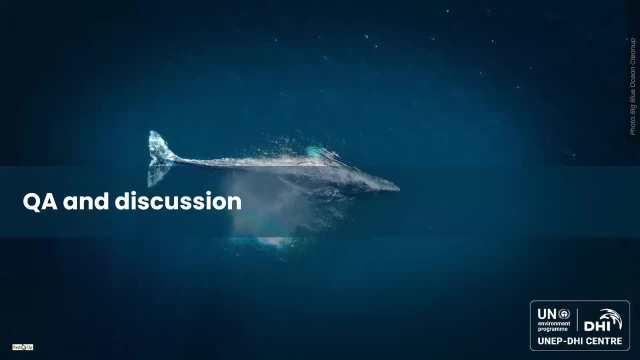 within your country. In many cases, there are a great number of entities that are doing different types of work within a country And there might not be the connection between the different stakeholders and the opportunity for the country also to have data and information available in one location. 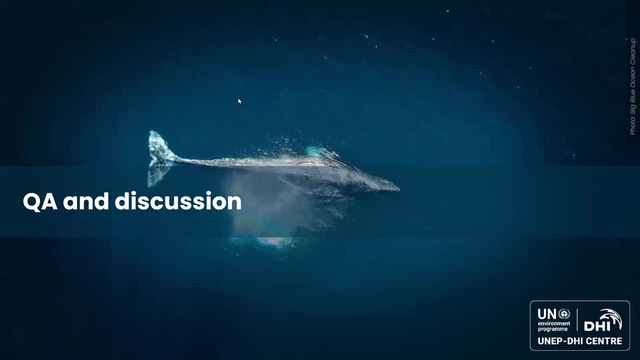 or being aware of all the ongoing work, but also the planning, what's in the pipeline. We're focusing on SDG 6,, SDG 11,, 12, and 14,, especially working closely with UN Habitat, as an example. 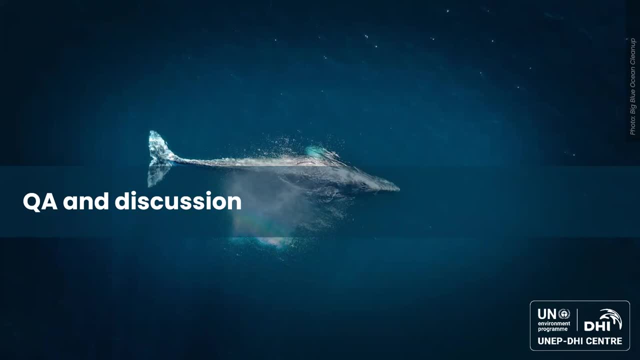 where we've been developing or supporting their development of the WasteWise Cities tool as an example. So here you zoom in on a city, you look at what's the situation, what are the waste flows at city level? what's the fraction of plastics? 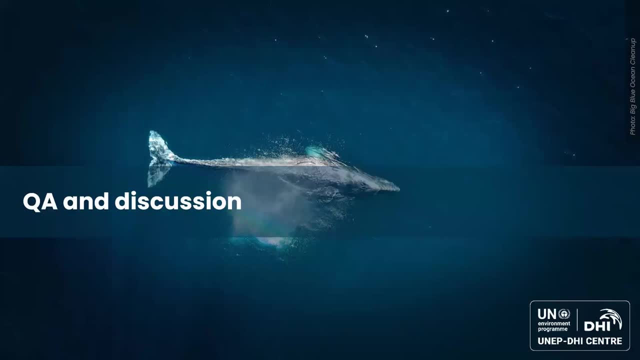 and you also have discussions with different stakeholders on what are potential modalities that would work best at the city level. This type of information can then feed into development of project proposals where you have the data, you have done the consultations, you have identified potential solutions. 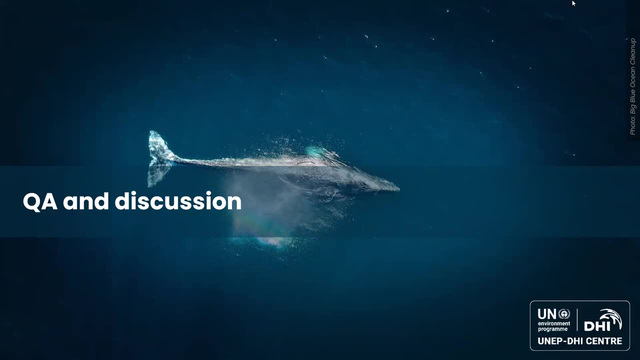 and you're now looking more for an opportunity to work with a partner that could help you to take those forward, And this is part of then. one example within an action plan that could be considered to address the topic on, for example, 11.6.1,. 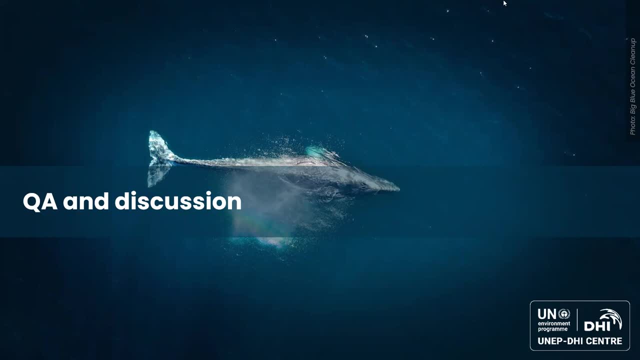 environmentally sustainable waste management And I think, for example, in Mombasa, where we then supported the implementation of this work with Habitat. then there were also follow-up discussions and proposals developed by Habitat, for example with, I think, EIB. 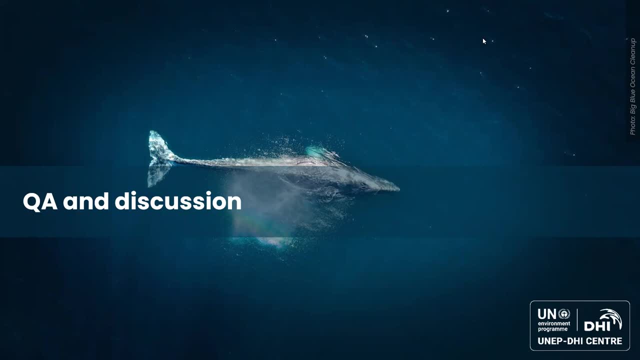 So it's more of an example on how we can help, through this process, connect the dots, identify the gaps for data, but also identify and support the management of data to identify. where do you want to focus efforts? where would a country wish to put their efforts? 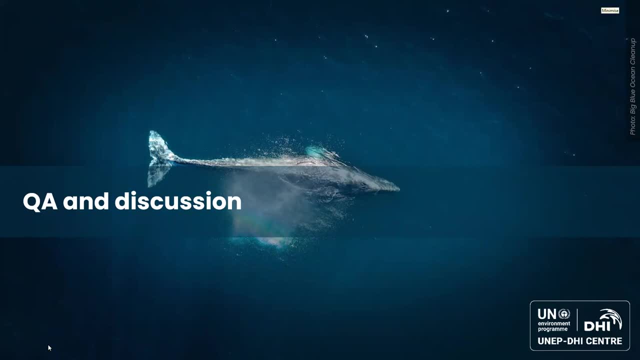 and what are policy-related efforts or legislative opportunities that they may wish to consider. It might be tweaking an existing legislation, it might be putting something else in place or seeing what options are. So that's an example of how we're approaching the action planning at national level. 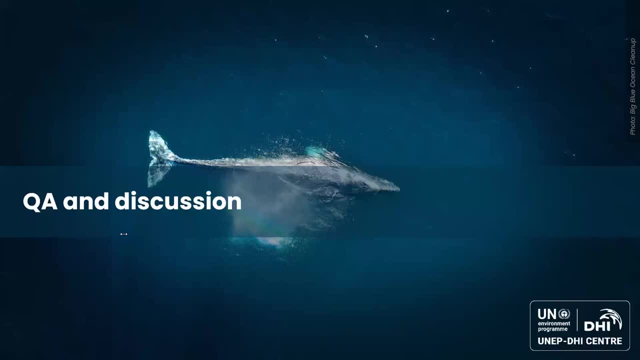 That's great. Thanks so much, Heidi. And, as you rightly mentioned, within the plastics domain there are so many stakeholders to look at And with that I wanted to turn to you, Karl, and just ask a question in relation to the GPML activities. 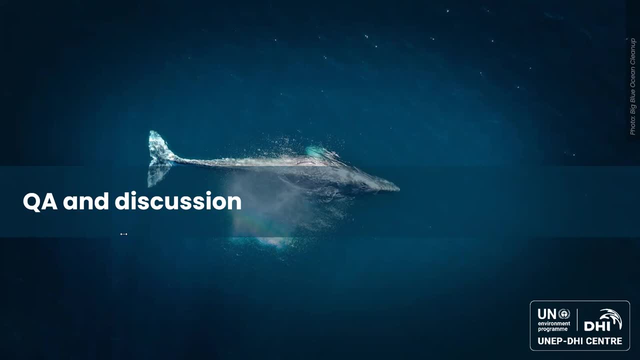 Of course, we're talking about stakeholders. We're also talking about partnerships as one of the things or one of the themes of this webinar. So I wanted to hear from you, along these various tracks, If there are partners out there, organizations that would like to engage. 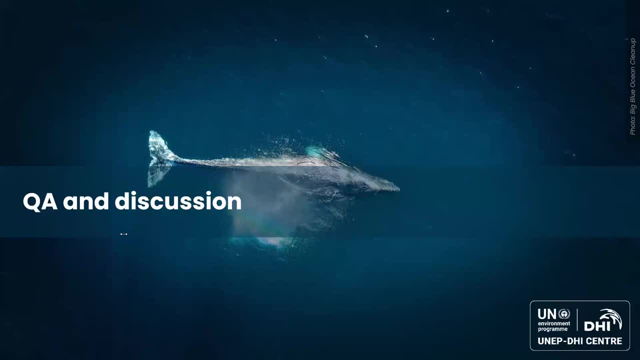 is there a formal process or what opportunities do they have to actively engage and become part of this GPML network? Yes, thank you. I shared and maybe I can put on the link too, but people are going to have access to the slides at the end. 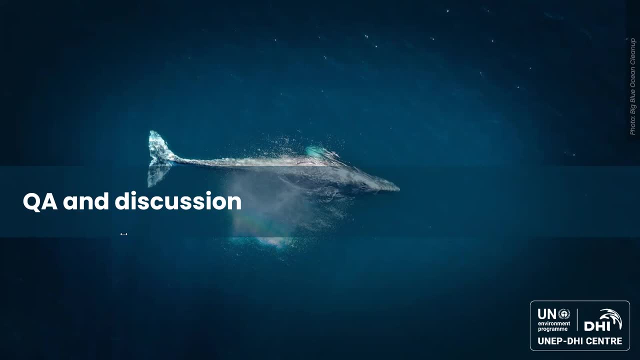 So I shared The Global Partnership on Plastic Pollution and Marine Leader is always inviting new members to join, So the partnership itself. the members are entities, so it's government entities or organizations, NGOs, private sector entities, And we welcome very much others to join in. 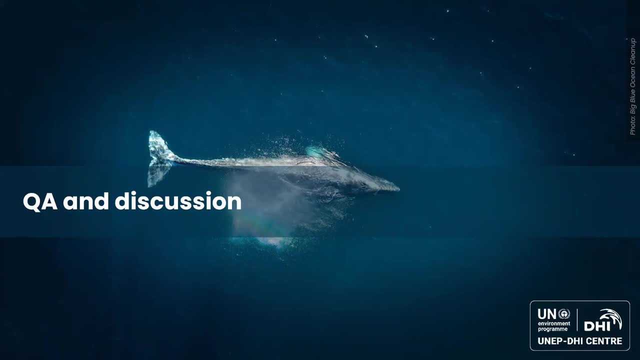 and to look at these five action tracks. I mean we're really the partnership. throughout its 10 years, history has worked on a range of issues from source to see really looking at, yes, preventing plastic pollution and marine leader from entering the environment. 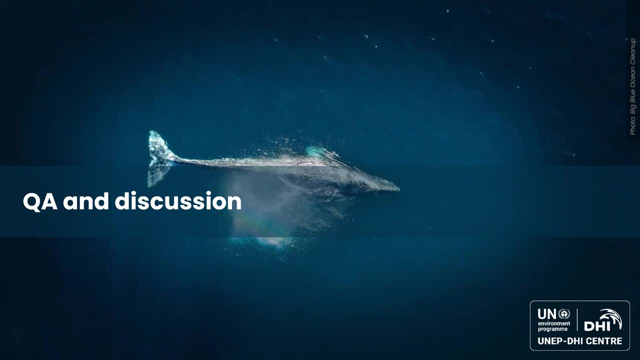 but doing so from a full life cycle perspective, right And from source to see in many ways. So, and also the other opportunities to join the GPML digital platform that can be joined by entities or individuals. And this is you know, it's still in its beta phase. 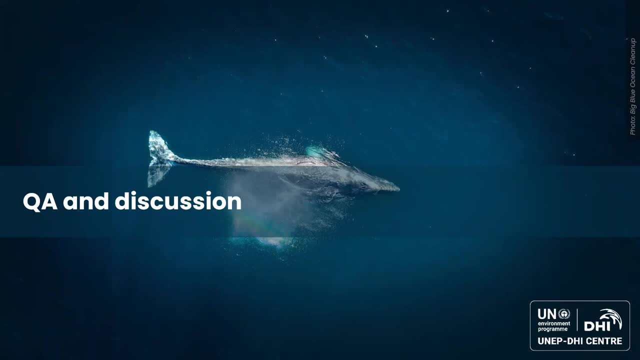 It's been developed since 2012.. It's a very robust, I mean. I really think it is going to be a very useful platform, not just for sharing information, but really for collaborating, coordinating. So I really invite you to join it. 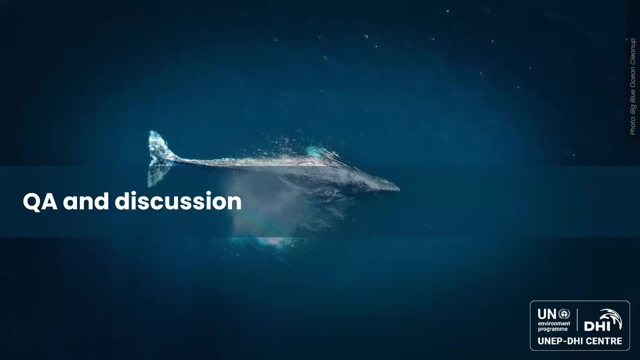 and to provide information. I mean, you've seen there's a lot of data partners et cetera to really utilize- provide information, but also really utilize this platform to further engage, And I'll try to click the links to both in the chat box. 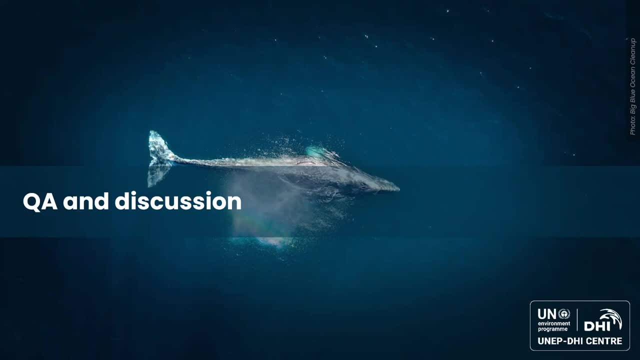 That's great. Thanks so much, Carla. And yes, we'll definitely make sure the links and the presentations are available. So just to recap again: everyone is welcome. There are plenty of opportunities. There's no sort of very formal process of getting to be part of those partnerships. 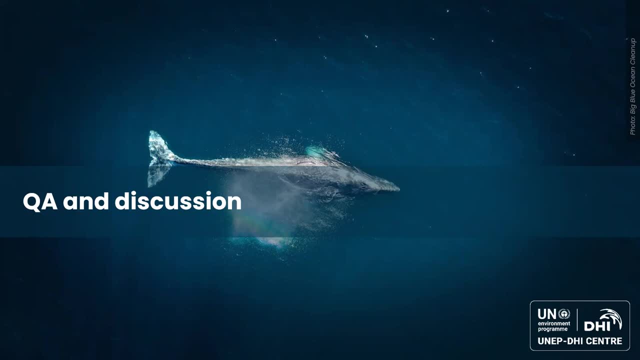 Going over maybe also to the data part that you referred to, Carla, and also Heidi. So question for you, Nicola, in terms of the digital platform, in terms of being able to, I'll give you a two-fold question, if that's okay. 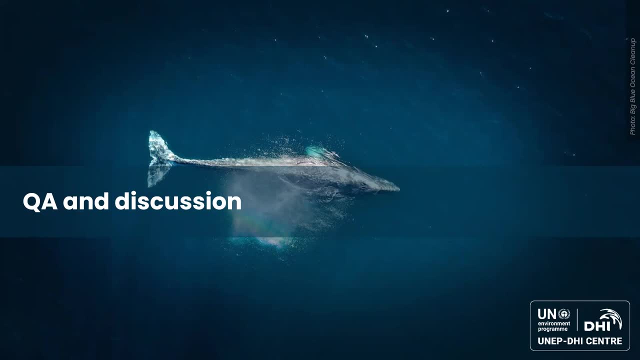 One would be in terms of being able to contribute data. if there are organizations that really do have global, local data sets, if you could speak to what are the options to contribute to the digital platform, I think that would be great, And also if you have any perspectives for the next. 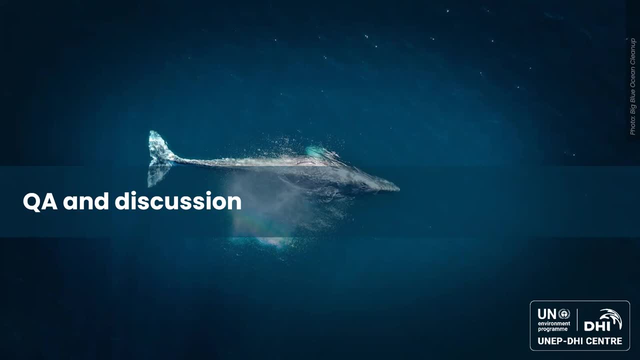 let's say two, three years. in terms of where do you see are the biggest opportunities for global data sets and also maybe the biggest needs or gaps in the data that are needed to support and inform the national action planning processes. your inputs or initial thoughts would be really welcome. 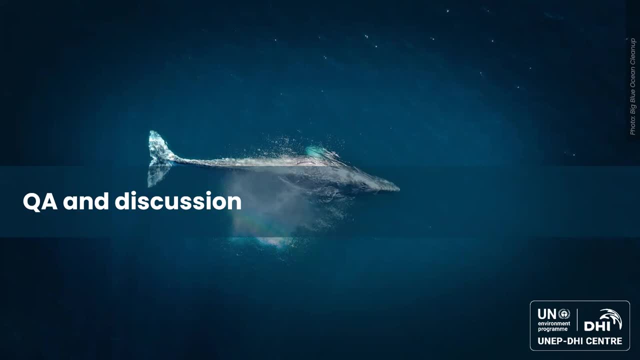 on these two. Thanks, Nicola. That was a long question. How much do we hesitate? now? We have a few minutes You can initiate and then we'll see if we have time to roll up. Thanks, Nicola. So maybe just to start with the first one. 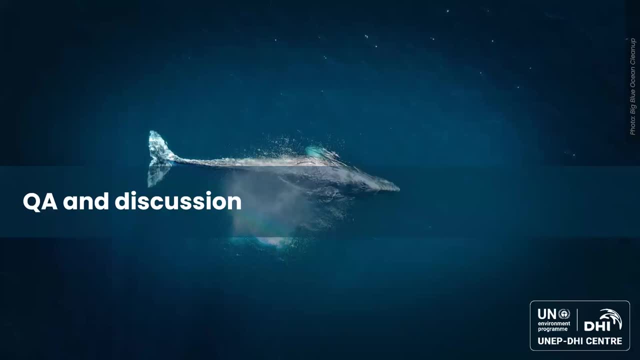 Yes. So we welcome very well- And I think this came from probably both- what I was saying. also Carla was saying. So I think, from GPML side, from our side, we're super happy to welcome the contribution from anyone who would like to be involved. 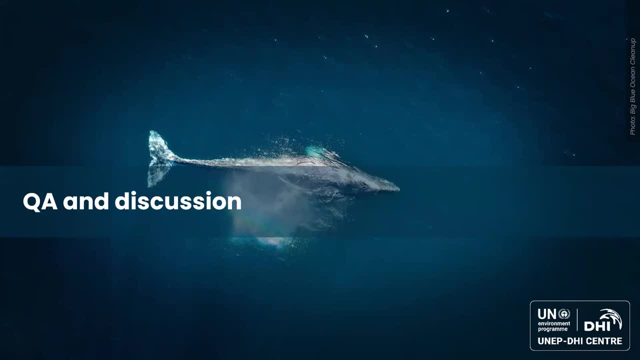 There is the opportunity to share data. So I dive a little bit more deep into some of the, you know, harmonization and all of this, but it's actually just possible to share data through the platform. So that's definitely something that we value a lot. 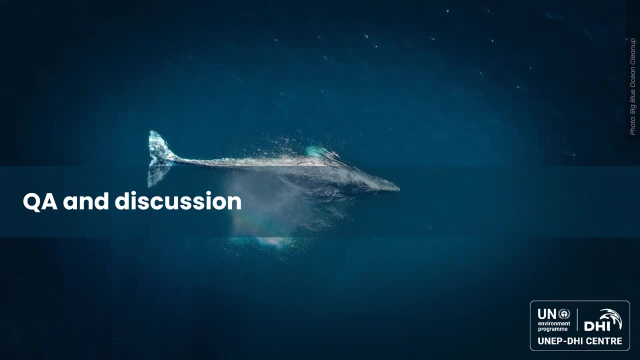 And if there is anything, you are, you know, any of you like sitting there and think like, oh, I've got this great information I would like to share with the rest of the other people working to deal with plastic pollution. of course, just reach out to GPML Carla myself. 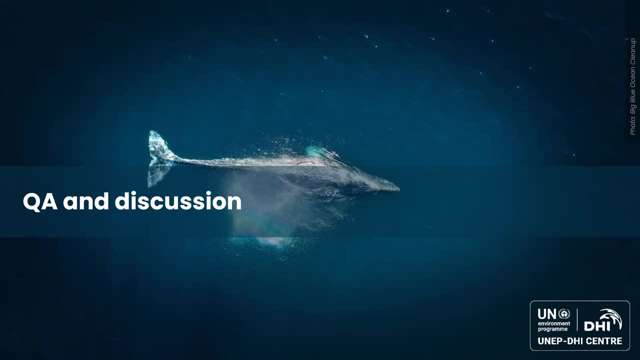 Heidi, and of course, I'm very happy to follow up and help you do that. Then, regarding, I would like maybe also to tap in. I could see, like Maya, you mentioned global data, but also local data, very welcome. 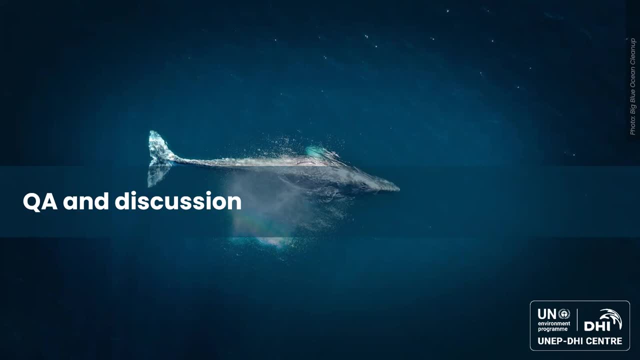 Because it was one of the comments in the Q&A around- like local data at the country level. All of this is, of course, very much welcome And it's great because it's something that can really support and strengthen some of the data sets that we have. 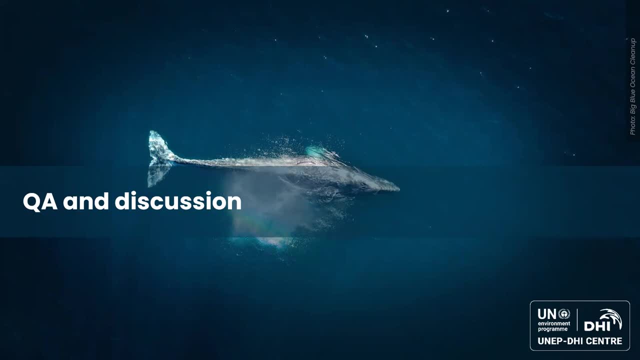 you know that are already there, Like, for example, also on the freshwater side, which is the one I gave a bit more closer example. Of course it's a global model, but we are looking, you know, more locally to kind of like strengthen. 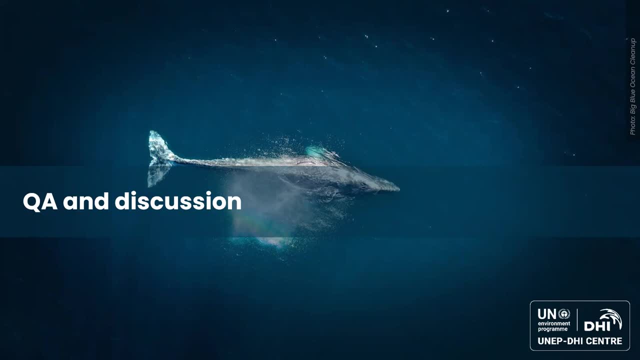 that data set and the information that have been used to create those estimates. Now, looking at broader gaps, that one is a really tough one And I think it will depend- I think, a lot also, I think- where you are operating. 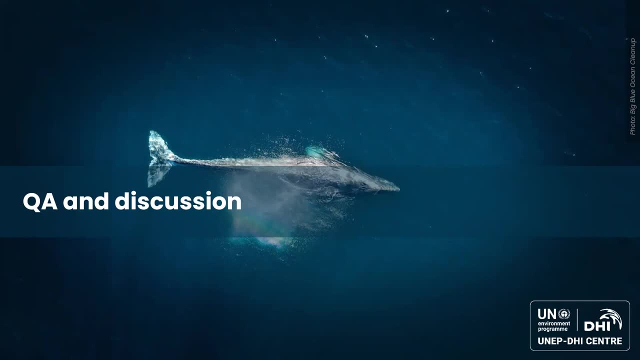 So there are some areas where, of course, the level of data accessibility is higher than others. I would definitely mention the one around the freshwater. that has been at least some of the action plans we have been seeing. It was actually, I think, one of the areas where we could see. 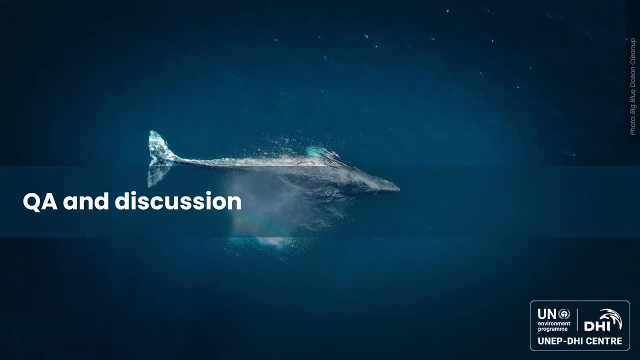 that there is an opportunity to strengthen that further. But I must say there hasn't been really close dialogue yet on the work that's been done so far. So I definitely see there an opportunity. But I would maybe also give- I don't know if we are allowed- 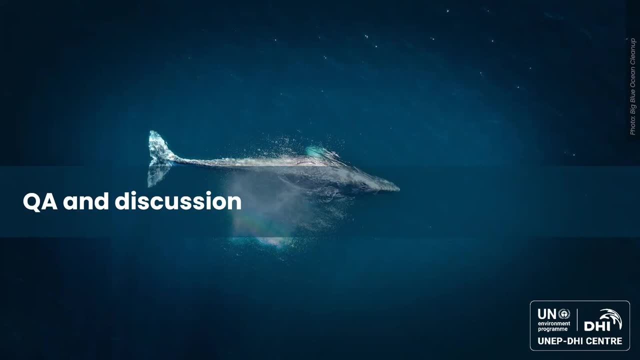 Maya, maybe also Heidi and Carla here could chip in. I'm sure they have a Yes. Thanks so much, Nicola. Let me just move over to Han, if that's okay. We have a few questions. I think that pertain very much to your presentation, Juan. 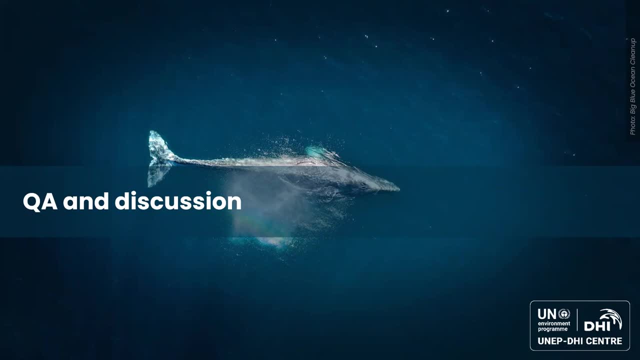 And these are actually from local stakeholders in Nepal and Sri Lanka. One, of course, would be: you know how do projects or potential initiatives could gain access to the funding from the initiative and if there are any criteria? But we also have two questions in relation to you know. 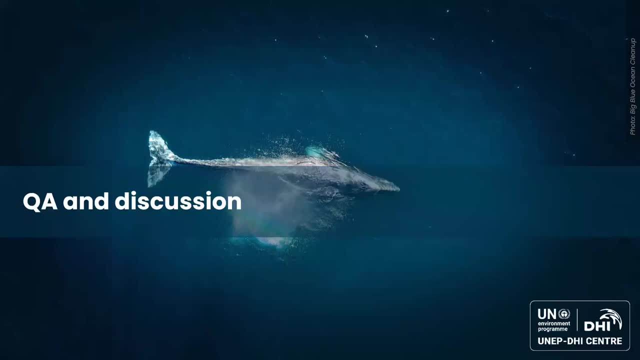 really opportunities for collaborate, For example, smaller pilot projects working together with local governments or local authorities. As you mentioned, there is underrepresentation of projects in Asia, for example. So we have a question here from Nepal and from Sri Lanka And you know if there are local organizations. 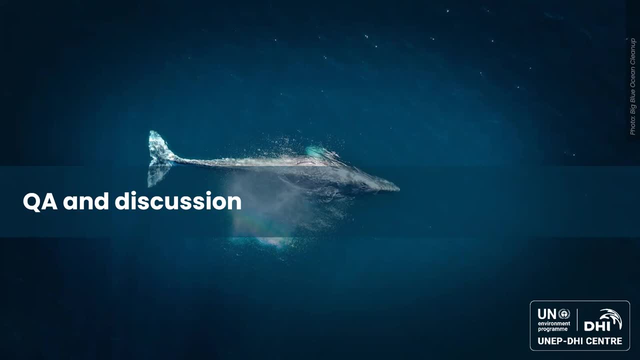 local governments, authorities, could they approach the initiative for collaboration And if there's any kind of process or your suggestions on that? Thanks so much. Okay, thank you, Maya. Indeed, both questions are related Because the way we try to find projects. 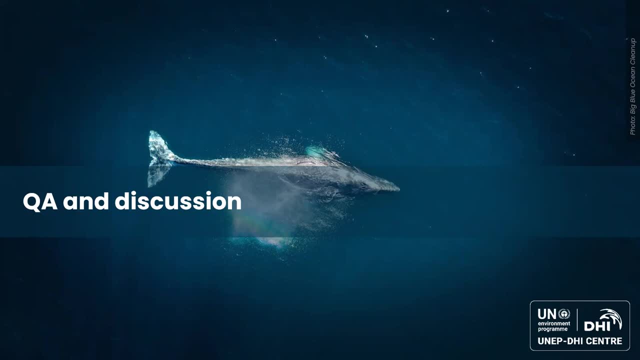 and prepare the projects to maximize the effect of plastic pollution is through technical assistance. We have right now one facility for Sub-Saharan Africa, managed by a colleague in the AIB, And what we do is that we have hired a consultant with a very high budget in order to find and prepare projects. 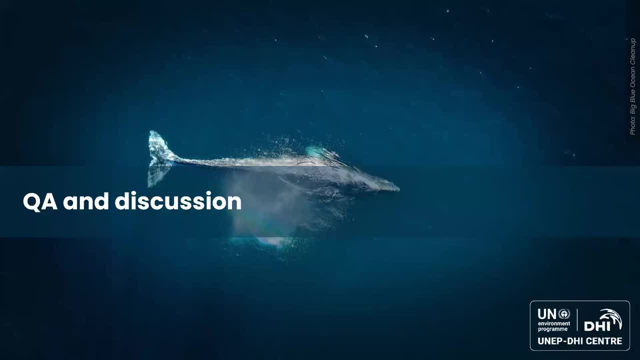 that are relevant for the Clean Oceans Initiative And these projects will ideally have pilot solutions in order to that these solutions can be replicated in other future projects, That's for Sub-Saharan Africa. So this consultant already hired. they are contacting governments. 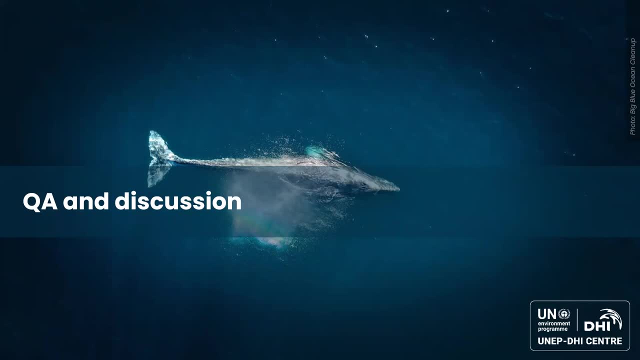 they are contacting other financial institutions or other stakeholders in order to try to find the best possible projects for the AIB and other partners in the Clean Oceans Initiative or other institutions to co-finance. that That's for Sub-Saharan Africa, But we are working also in a similar 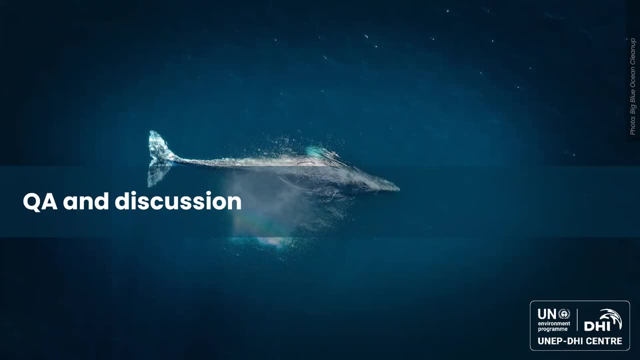 similar facility for the Caribbean that will be in place, likely in March, sorry in May, June this year, That one. the idea is also to find up to six projects with also pilot and very, let's say, targeted contribution to oceans. 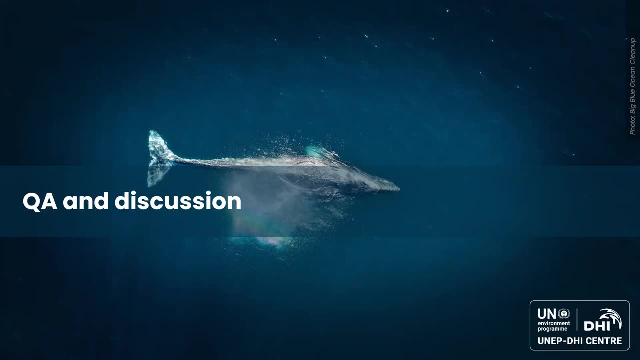 Also with some possibility of grants. if the part of the project is really relevant for the- as I mentioned before, if it's really relevant for the objective, for the Clean Oceans Initiative, for example, then we can try to find to channel a small grant for that. 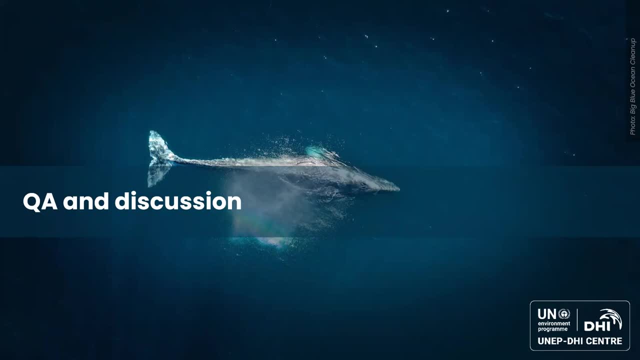 That will be in the Caribbean and we will start in June, And in Asia we're looking for something similar. Unfortunately, we don't have yet the facility. We don't have yet a facility, as I mentioned before, for TA, for identification. 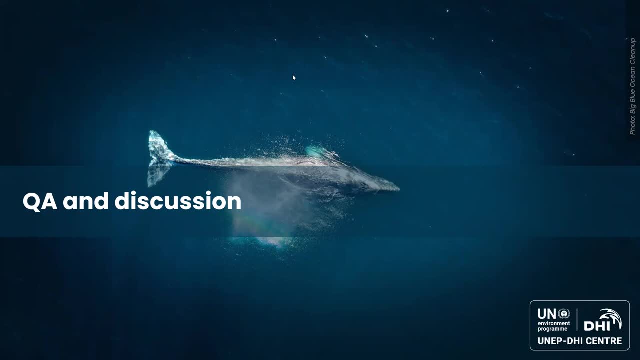 and also for grants that will also incorporate this consultant, Ideally in Asia. we'll try to find the projects and we also talk to the stakeholders, researchers and even, as it was mentioned in the question, and also even ideas of pilot plans or pilot solutions. 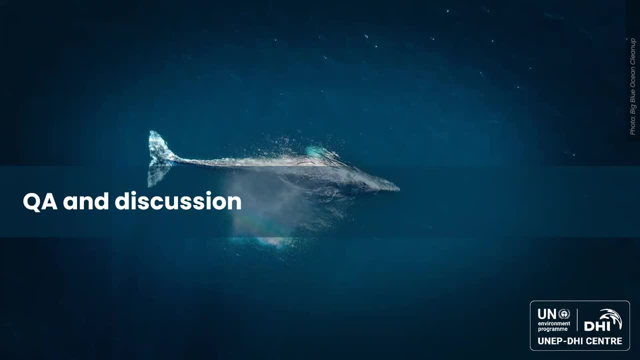 This Asian facility. we're in negotiations with the EU in order to that we can have it in place. It will call COTAF- We gave it that name- and it will be only for Asia, replicating what we have in Africa. 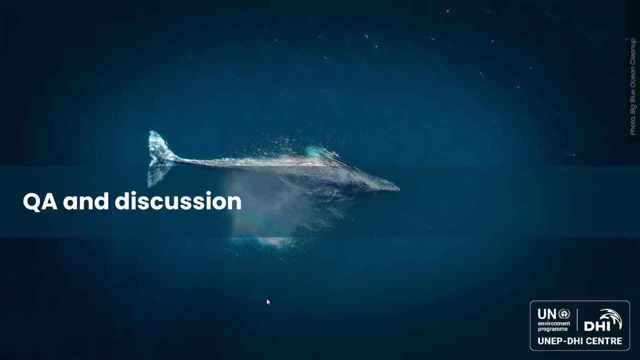 so for South Africa and in the Caribbean. So hopefully it will be in place and when it's done we will try to give try to give sufficient publicity. So, yeah, any ideas are really really welcome. Thank you, That's great. 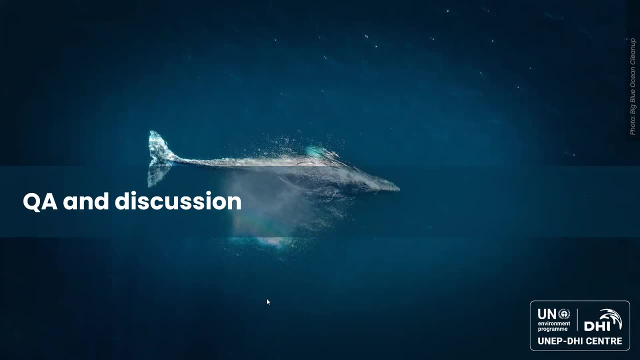 Thank you so much, Juan. So what I'm hearing is need to stay tuned. There will be. there are opportunities to be engaged. I'm afraid we have run out of Q&A time. We will pick up on any questions that are left in the Q&A. 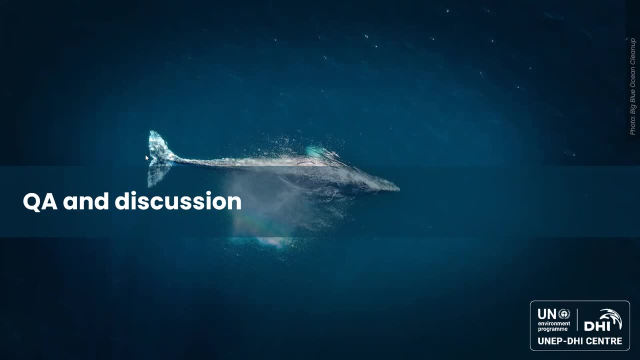 and see if we can respond to you offline. Otherwise, I would really like to thank all the participants and the presenters once more and give the floor to Louise for just a couple of minutes of closing remarks. Thank you all. Thank you, Maya.